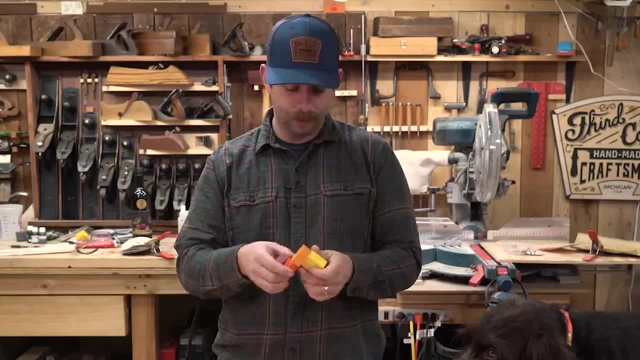 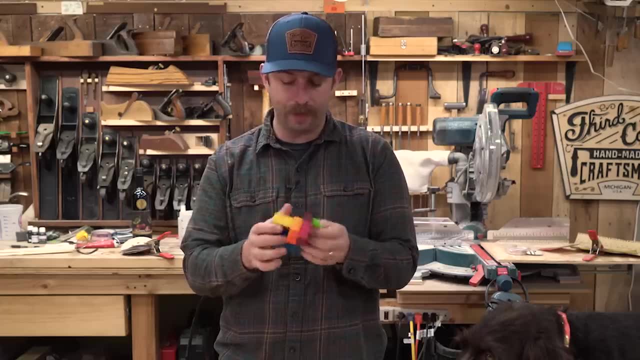 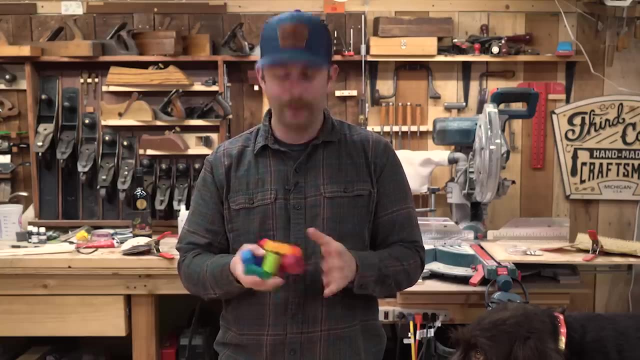 And then you can kind of pull it apart And it's just kind of fun to play with. It kind of morphs and spins inside and shuffles itself up, And then you have to kind of spin it back in place And well, you get the idea. 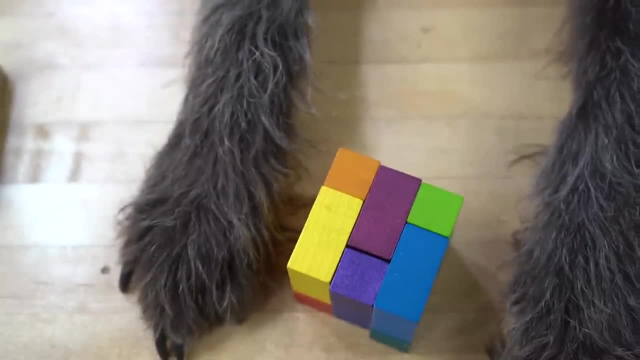 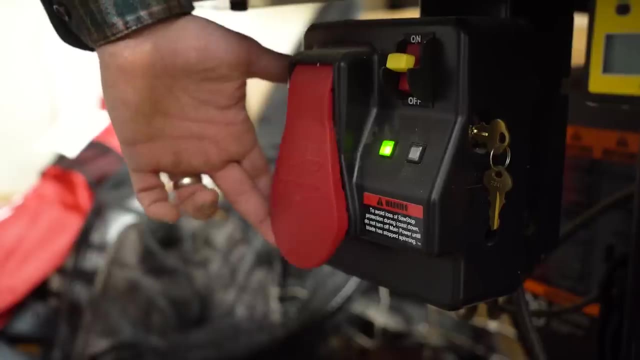 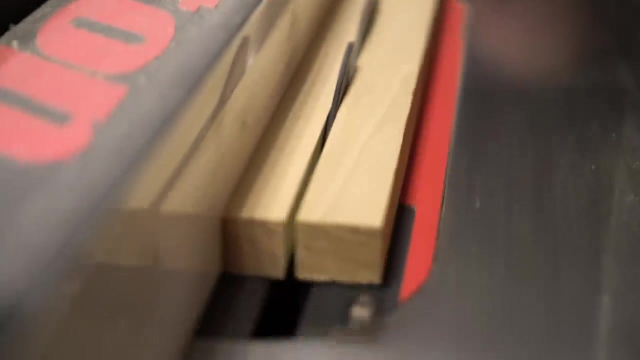 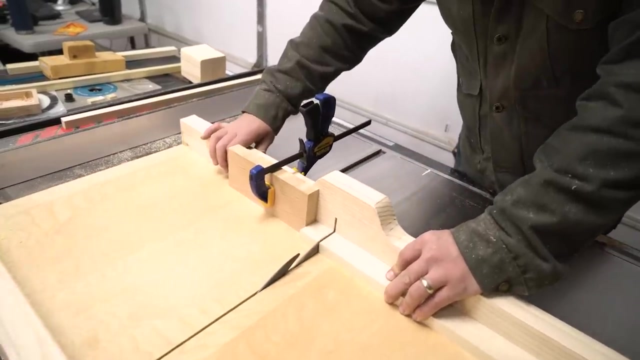 I'm going to use a three-quarter inch piece of popper for this build and start by ripping a one and a half inch wide strip and then a three-quarter inch wide strip. Then I'll set up stop blocks on my cross-cut sled, again at one and a half inches and then three-quarters of an inch I'll need. 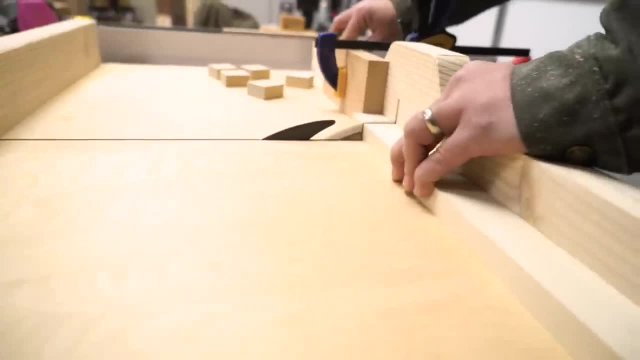 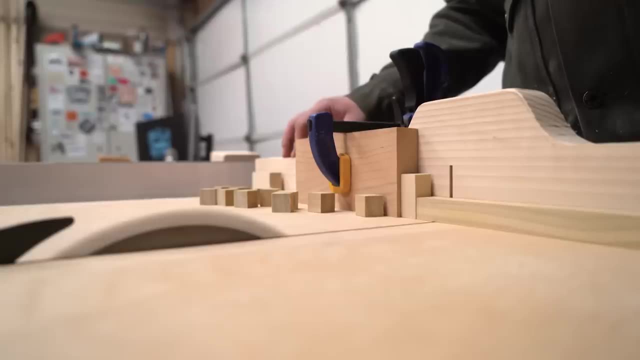 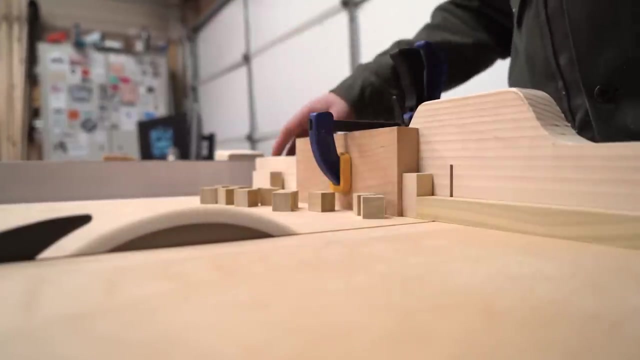 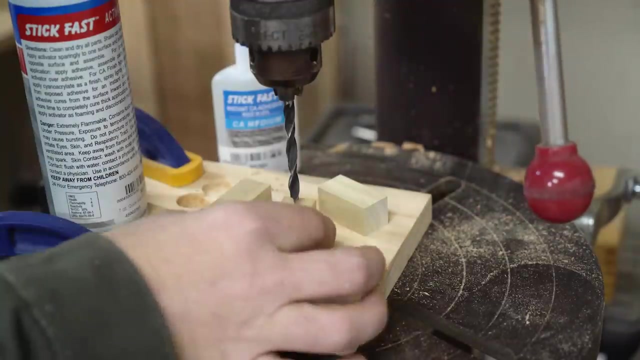 three of the bigger square pieces, six of the longer rectangular pieces and three of the small square pieces. I'm going to end up making several of these cubes as gifts. That's why you're seeing more than what I just mentioned. Next I'm going to make a quick jig to help me line up and drill holes in each piece. 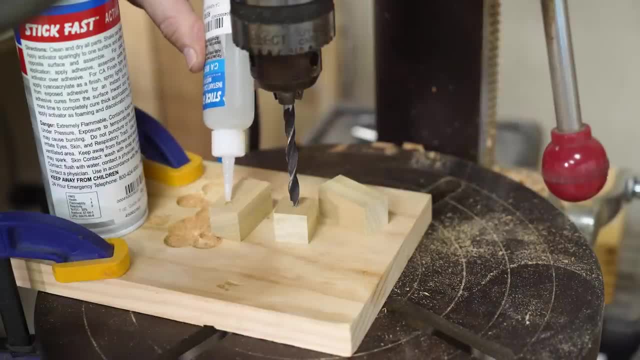 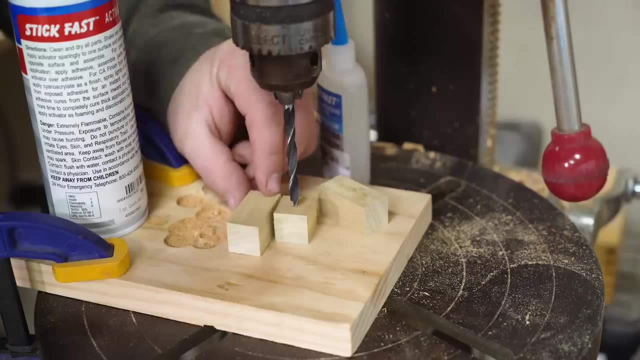 Each piece needs to be drilled in a certain way and I'll show that a little bit later on. But I just glued down a couple of scrap pieces with CA glue and I'll instantly cure those with a shot of activator. I like to use a. 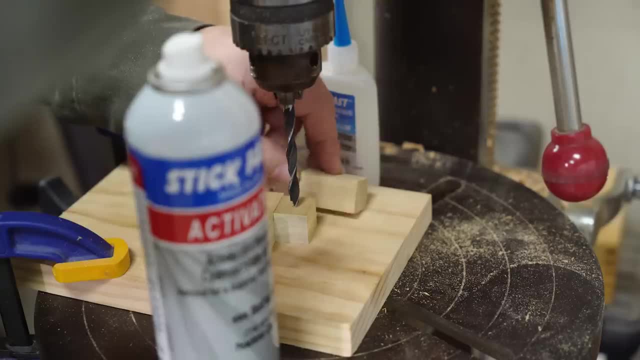 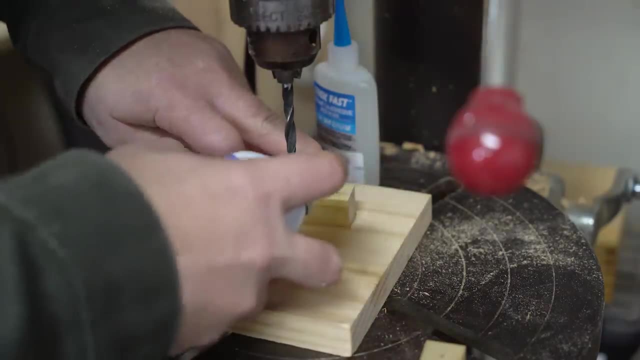 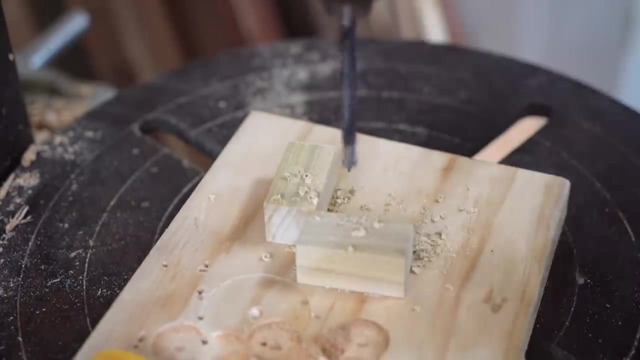 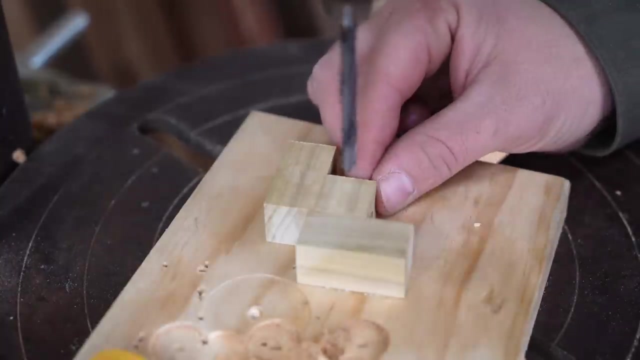 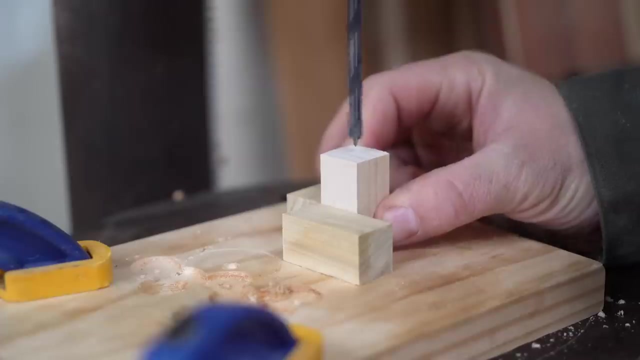 drill press for this, because I can set the depth stop so that my two holes will meet in the middle At around 35 degrees and 30 by 25. you should be doing the same thing. So here it is, Drilling hole. I'm starting on how long I'll make it when I end up making the end part of mylet. 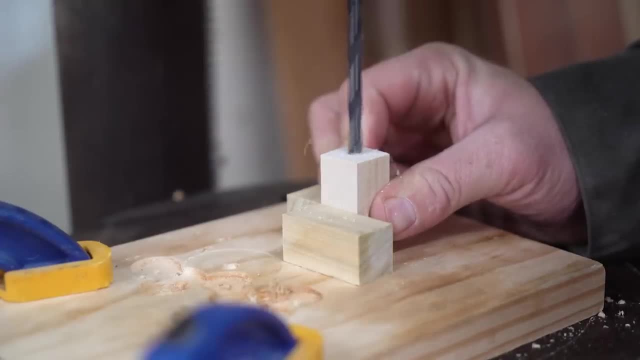 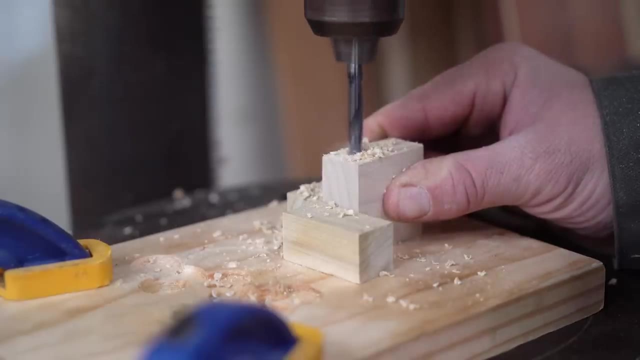 The��inash makes every piece of dough into five or six pieces so that it doesn't shift. I'm starting off with two pieces, One of myئ three and a half inches, so I don't hit a wall. that is 1.7 inches to the left. 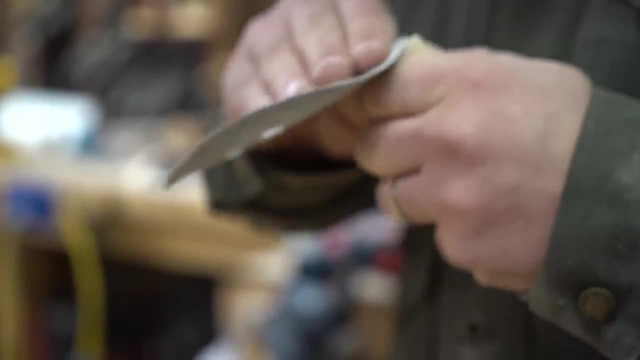 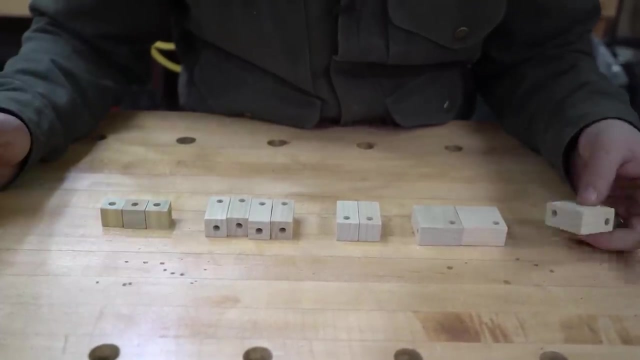 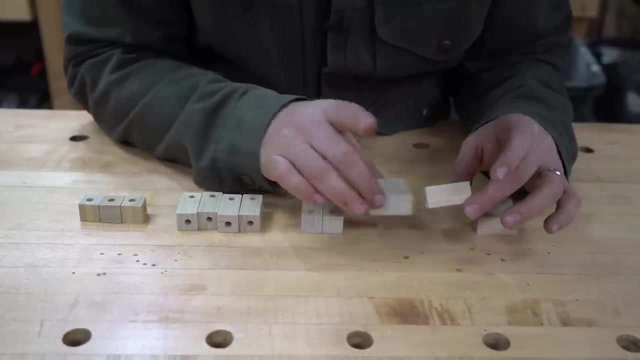 nee, Alright, so you need to drill the these holes in these pieces in a certain way to make this thing work. One of the square pieces you drill into the faces opposite of each other, so they meet in the back corner. The other two square pieces you drill one in the top and one 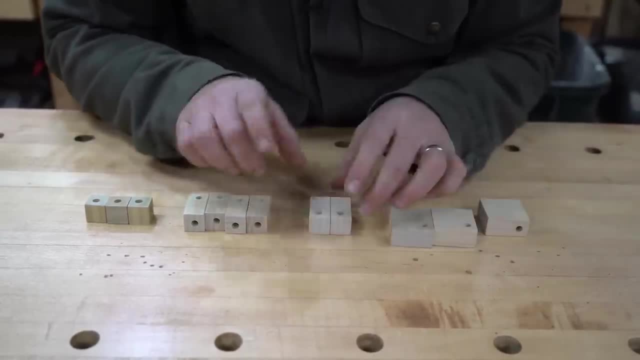 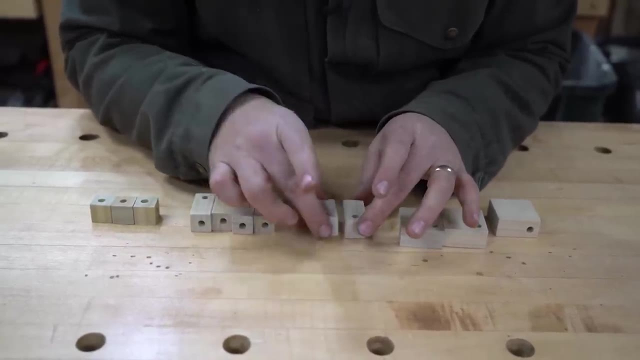 in an edge like that. Those two are the same. One of these longer pieces there'll be a hole that is drilled in two adjacent faces that meet in the middle, and four of the longer pieces there will be a hole drilled in one face and a. 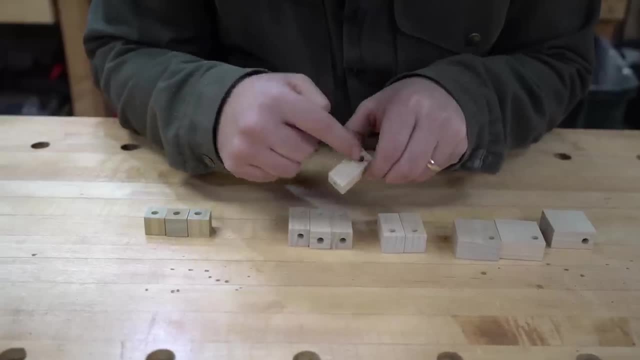 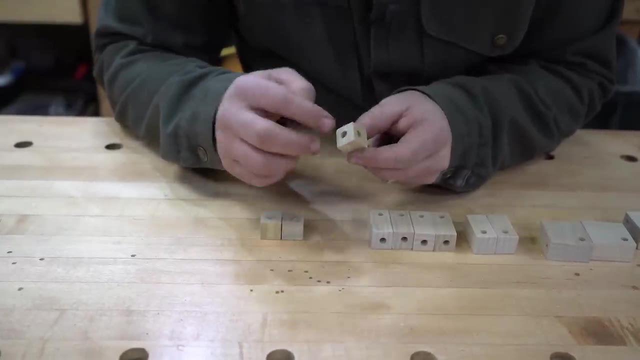 hole drilled through the end that comes all the way down and meets that face, and then the square ones, the little tiny guys. just two adjacent faces, so don't drill all the way through just any two adjacent faces. Alright, so we're going to put this together, but it has to go in a certain order. so I want to show you real. 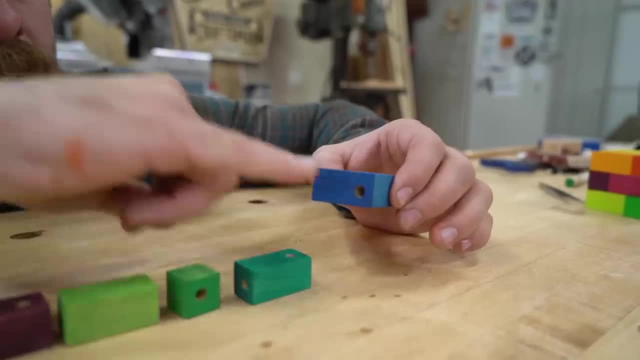 quick the order of operations. We're starting with the blue one. The blue one has a hole on the side and a hole on the top. The next one has a hole on the side and the next one has a hole on the top and the next one has a hole on the. 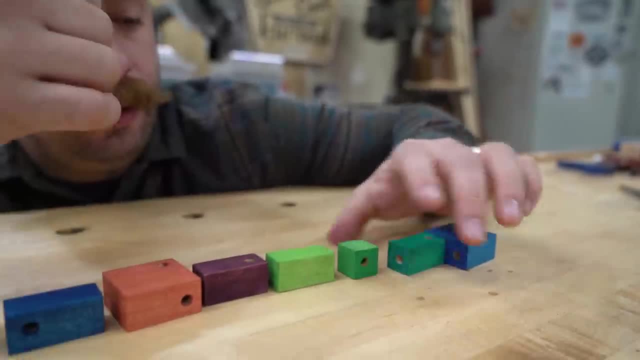 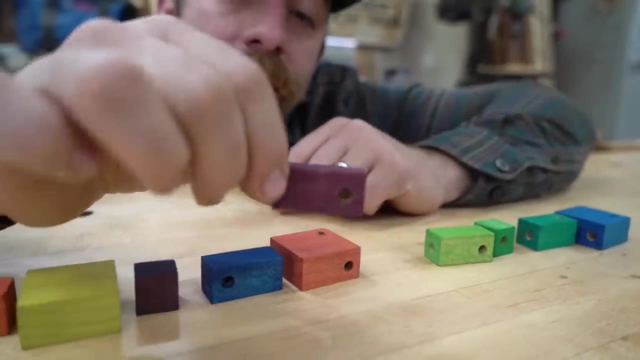 side, a hole on the end. The next green one is just a regular little square, doesn't really matter. The next one is a hole in the end, a hole on the side. The next one is two adjacent holes on the side: hole on the top, hole on the side, hole on the. 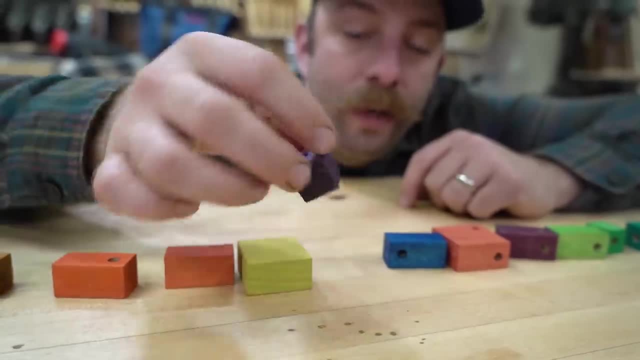 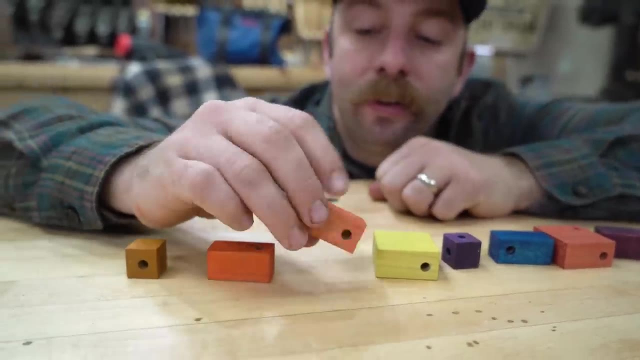 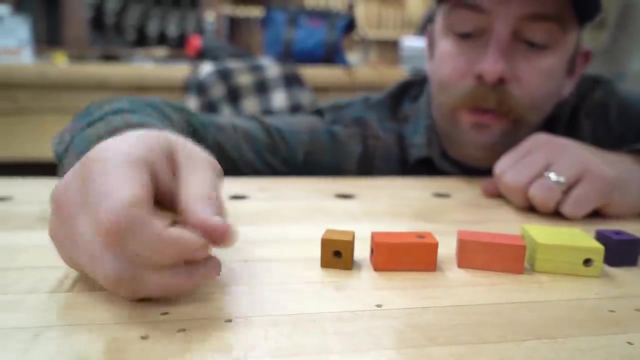 side hole on the end, Regular little square. This last one is two of the holes on opposite faces. Next one is a hole, two adjacent holes on the sides: a hole on a face, a hole on the end and then a regular little square. So I found this. 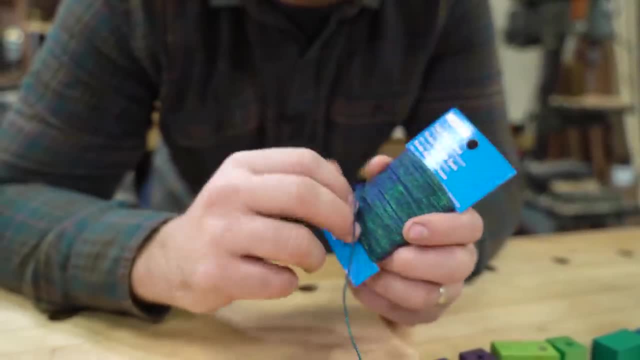 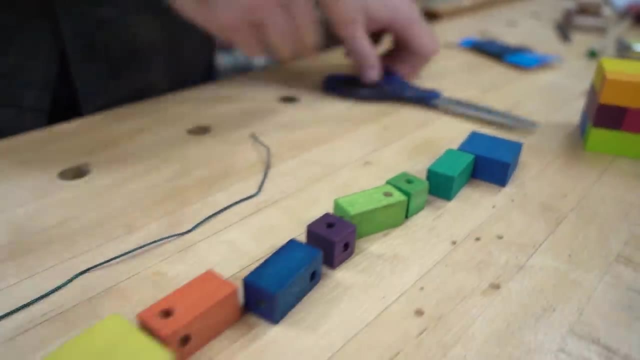 elastic cord. I wanted to find something a little more heavy-duty, but this is the best I could find. I found it at one of my local craft stores. I'm just going to double it up and pull it. really nice and tight and hopefully it works well. 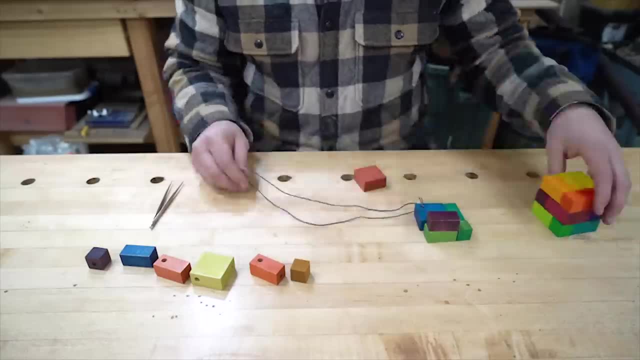 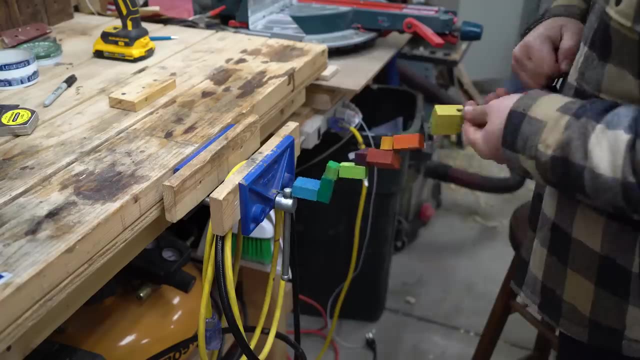 I forgot to mention that I painted these with watercolors and then I coated them with a semi-gloss Minwax polyurethane. I didn't get the color spot on like on the original, but I still think it looks good enough, And a pair of tweezers works great for fishing. 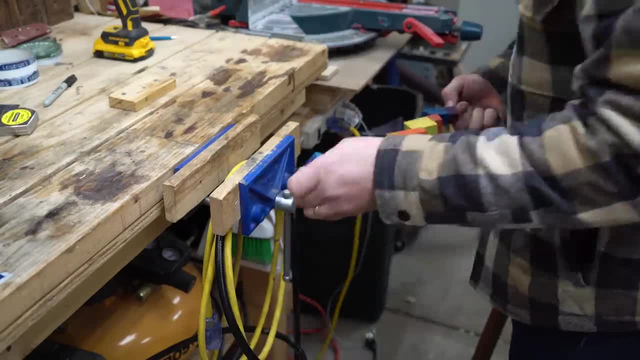 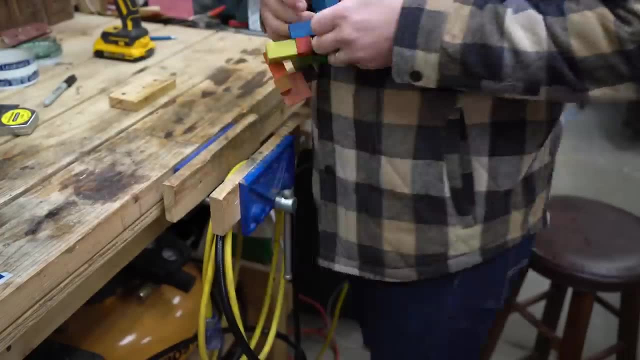 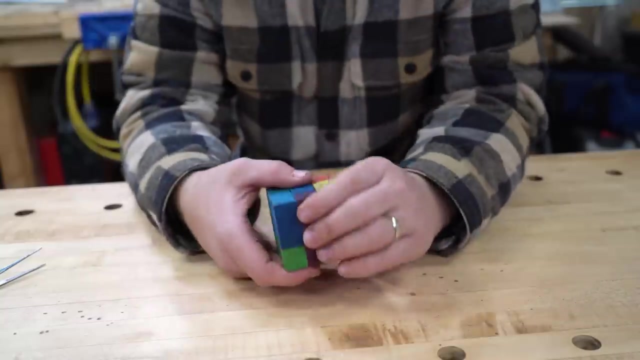 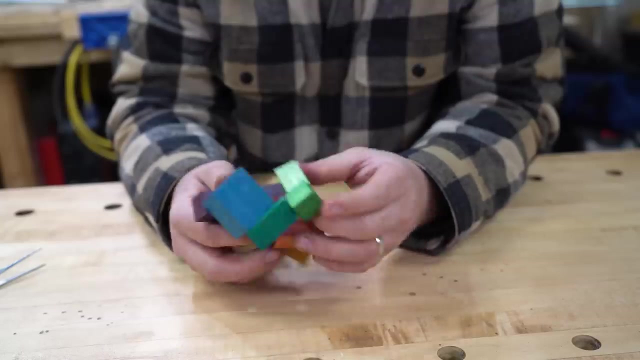 that cord through, Then I pull the pieces on the cord as tight as possible without breaking it, and then I tie the two ends together and I'm all done. Bingo. Now all that squeaks. really bad is that the tube comes right out of the 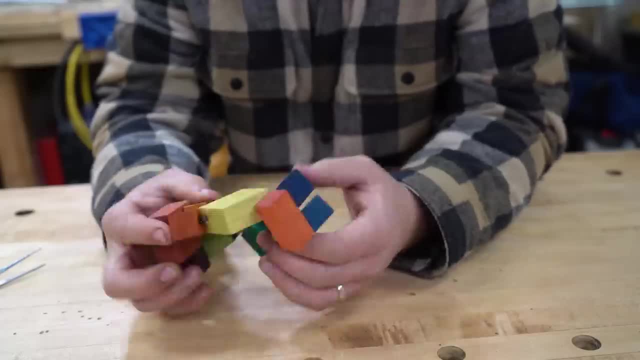 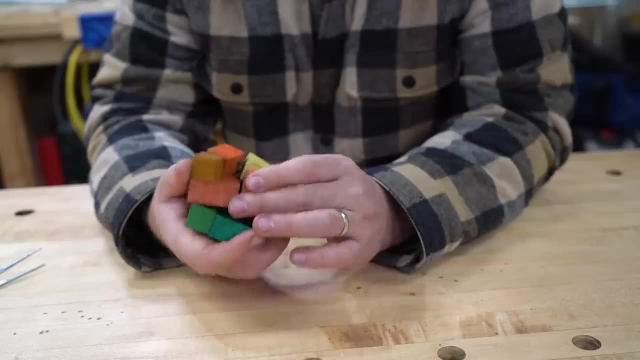 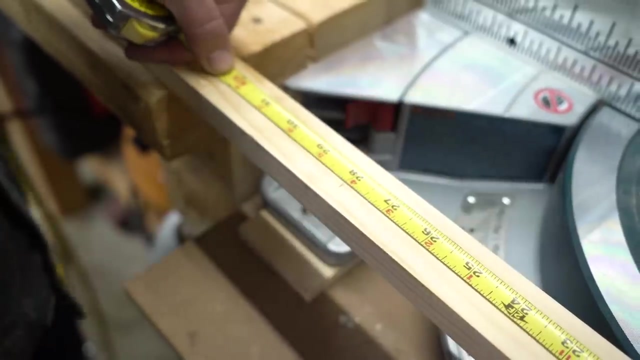 tube that you used to hold it there in case something breaks out. So I'm Obviously going to set up the old sìko says that it's upwards, So I can do that on my watercolors for the rest of the project. The next project I'm going to make is a little bath tub tray for my wife. I starts: Hey aún, så tìm để tìm, như im hằng tỷ để làm hình sẽ làm Mazem, первый đường kh Salvina và các đường ngồi của mình, Deborah. 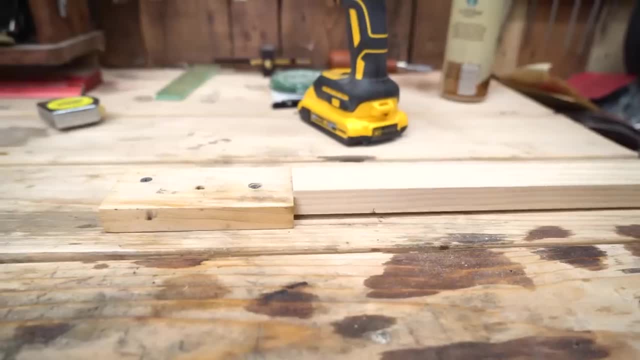 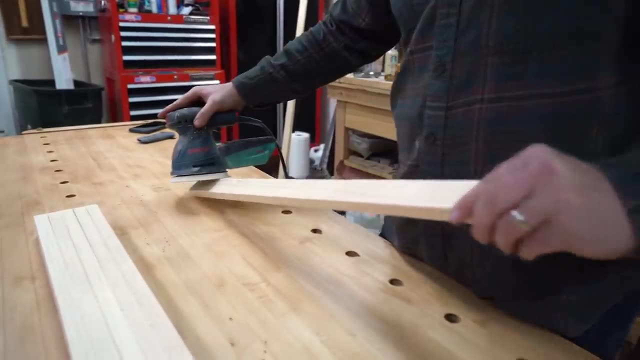 estáv с and a half inch wide premium boards that I got from Lowe's and I can just cut those down to 28 inches long, which is the width of my bathtub. You could also take wider boards and rip those to whatever width you want, too For this. 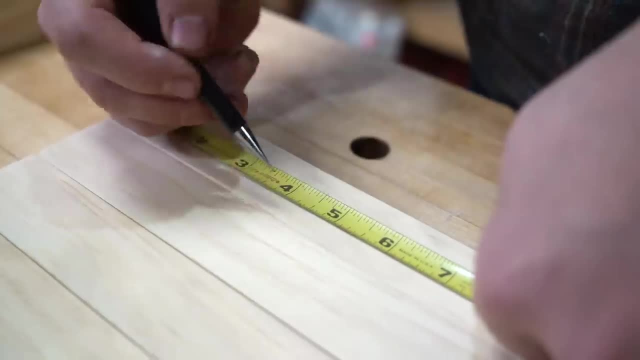 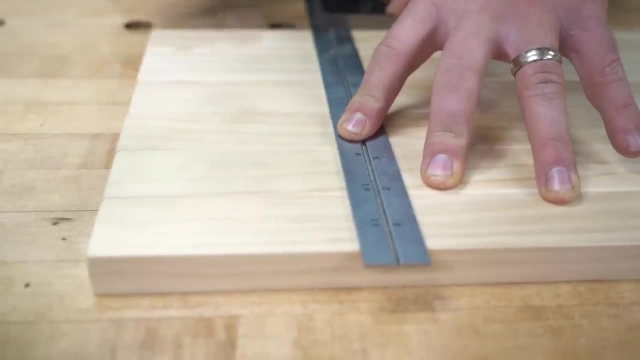 project. I would recommend working off measurements from your own bathtub if you want it to fit right. Our tub has a four inch lip on one side and a one and a half inch lip on the other side, so I'm going to screw my bottom cross members. 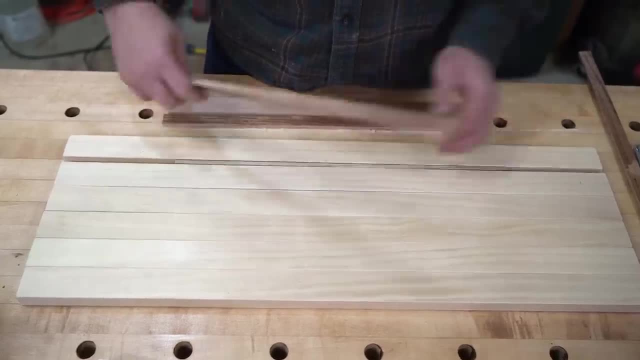 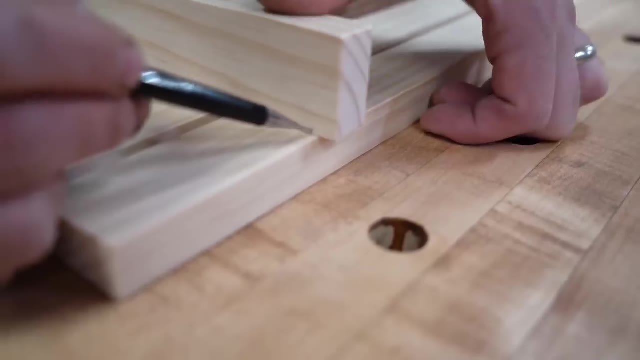 at those spots When the tray is placed in the tub. the bottom cross members will then lock into the inside edge of the tub and it'll prevent it from falling in. I'm using quarter inch pieces of scrap to make some spacers. then I'll mark and 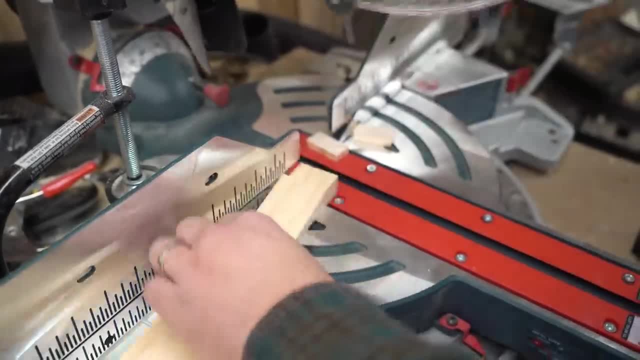 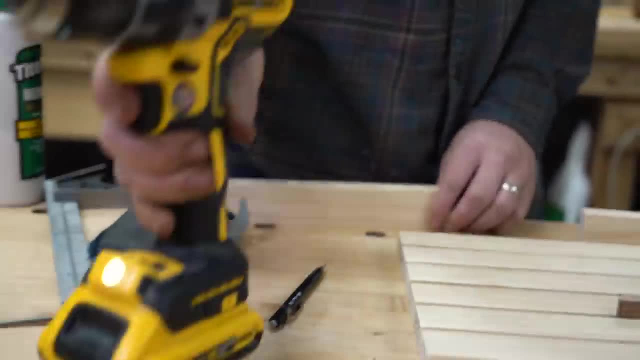 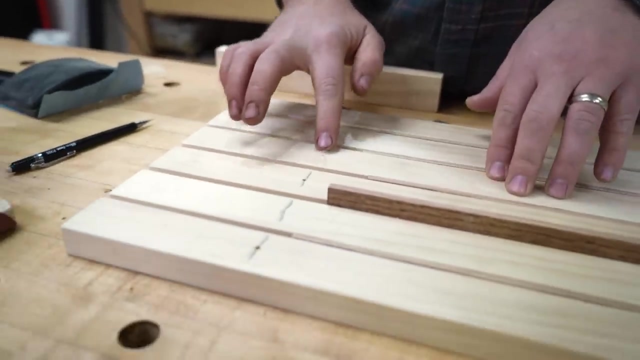 cut my cross members and screw and glue them into place. And if you like this video and you haven't already, please consider subscribing to the channel. and if you hit that bell icon, you'll get notifications when I post a new video. So thanks, so much for that. 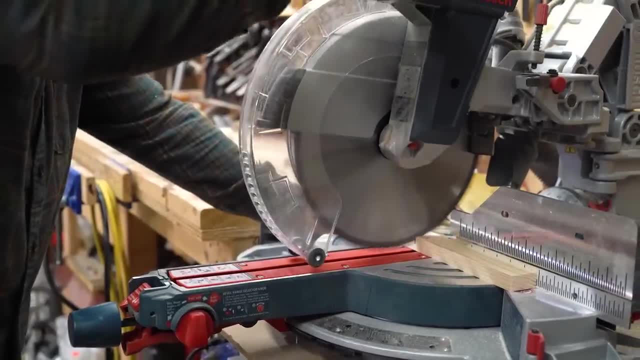 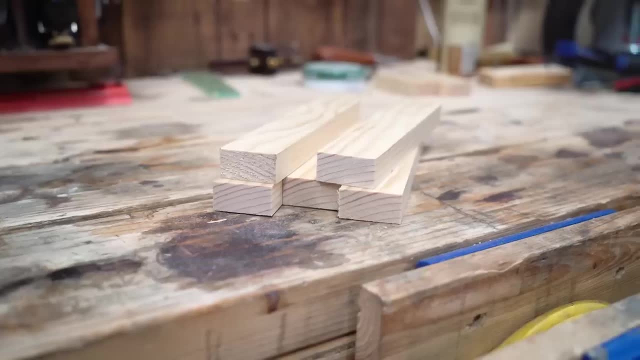 Next I'm going to make the book rest. The book rest will have six vertical slats that I cut at seven and three-quarter inches. then I'll use my cross members to make a cross cut sled on my table saw to make a three-quarter inch long tenon on. 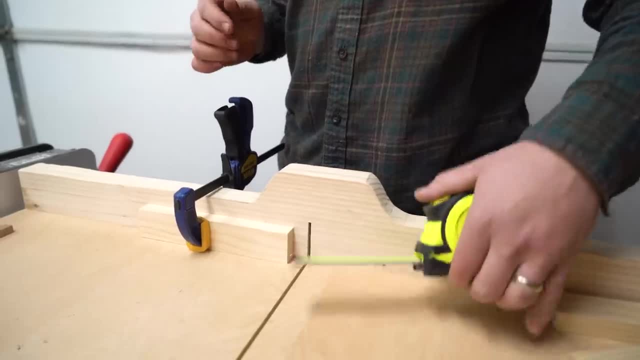 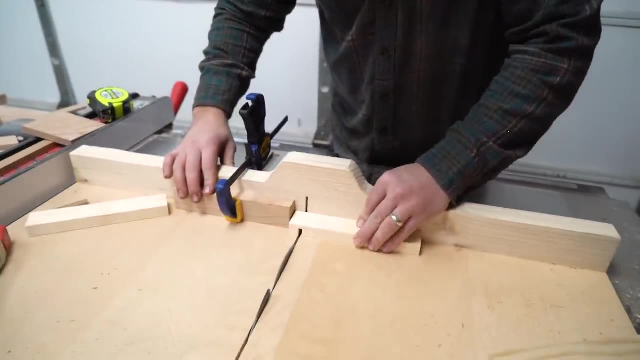 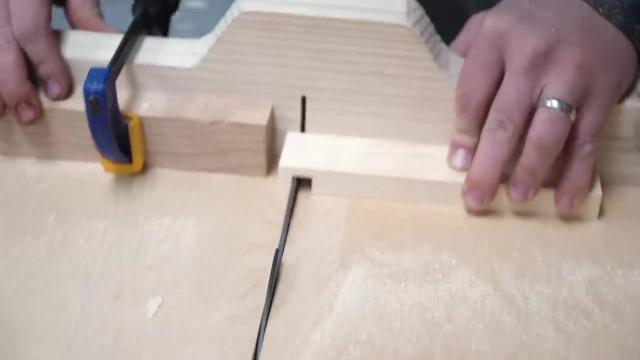 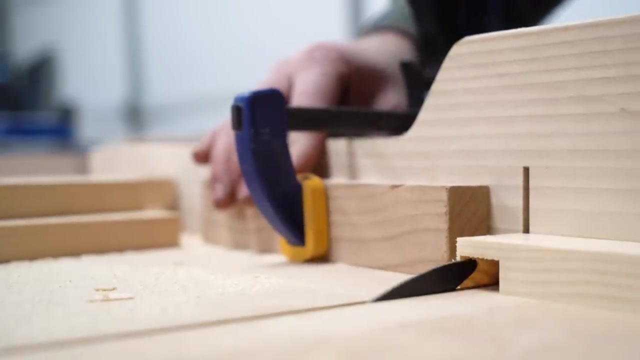 each board that is approximately a quarter inch thick, so that when I secure them all together the tenons on the book rest will fit into the gaps on the tray. so I'll just cut off two drops of this cross piece of scrap and then I'll screw in the 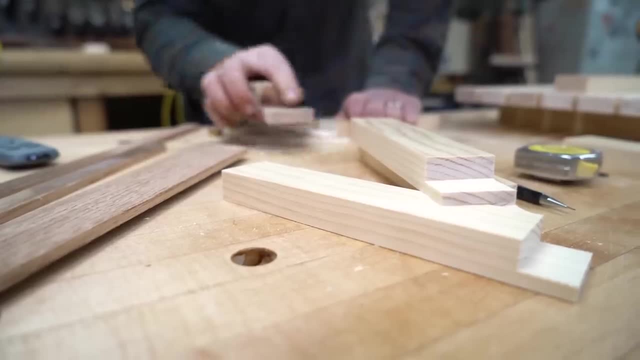 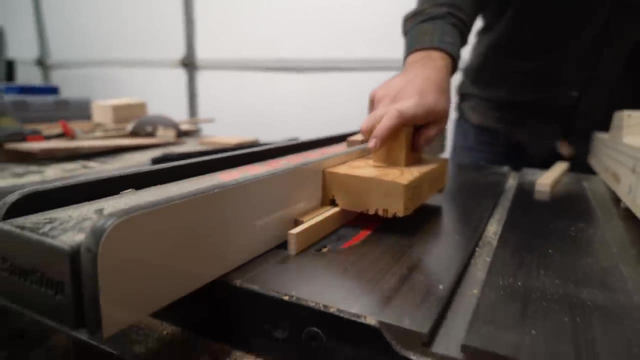 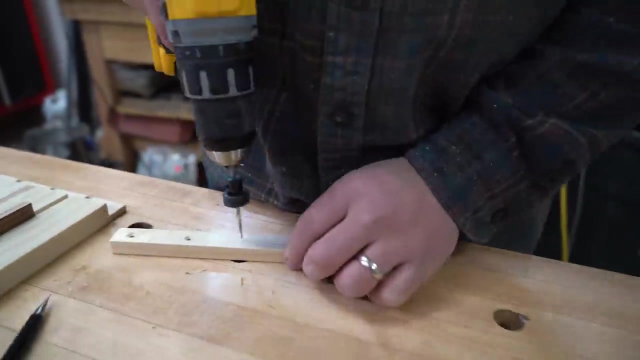 tenon. Now I'm going to make the second and third slats and I'm going to make a two by two slat. So I just cut it a couple of inches larger than the first one and then I'm going to just trim the slat off. 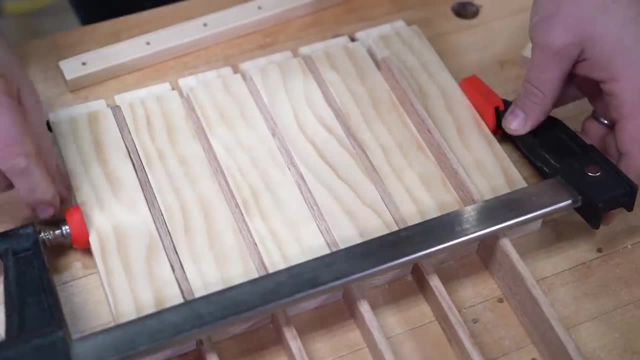 Now I'm going to use a clip. I'll just cut a little bit off, Simple as that, And I'm just a couple of half inch pieces that I'll use to secure that book rest. Now I'm just using a clean one. 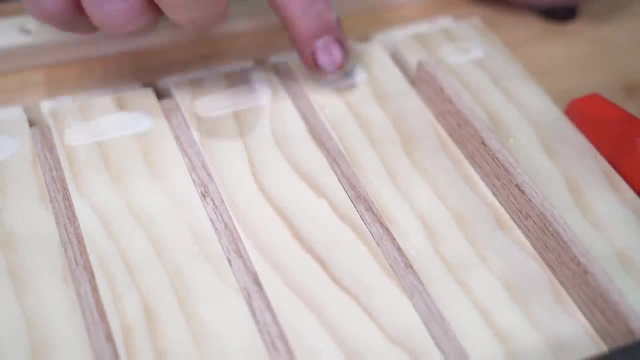 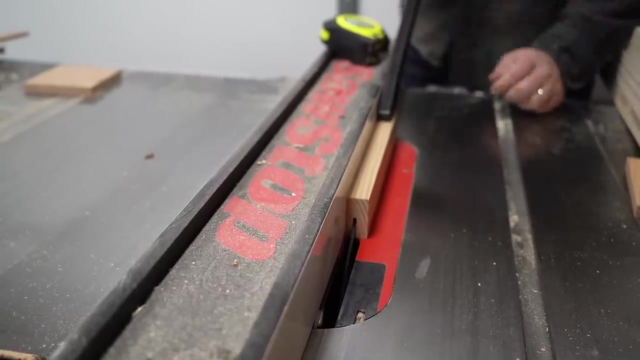 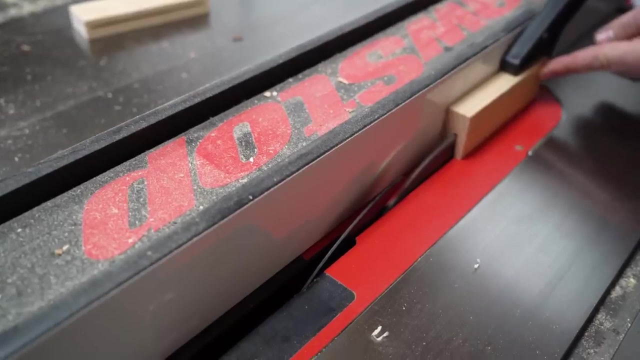 clamp to kind of hold those pieces while I screw them together. Now I'm going to make a little insert that will prevent the book or tablet or phone from sliding down when it's leaning against that book rest. I'm essentially just taking two rip cuts through this one and a half inch board to create a piece that. 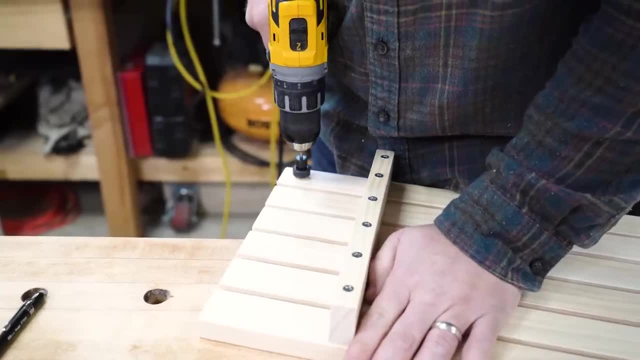 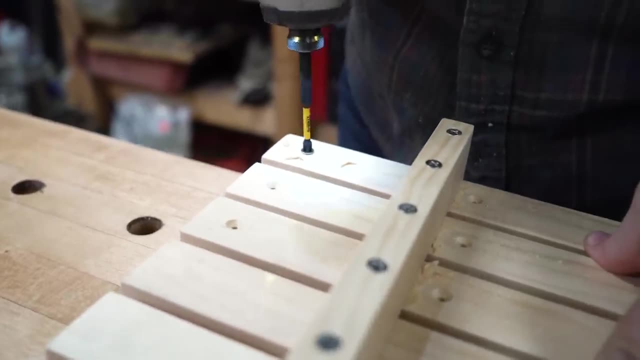 has a quarter inch rabbet that can drop into the gaps on the tray, Then I make two shorter versions of that and I'll just turn those on their side and secure those to the top by screwing through from the underside, and those will be. 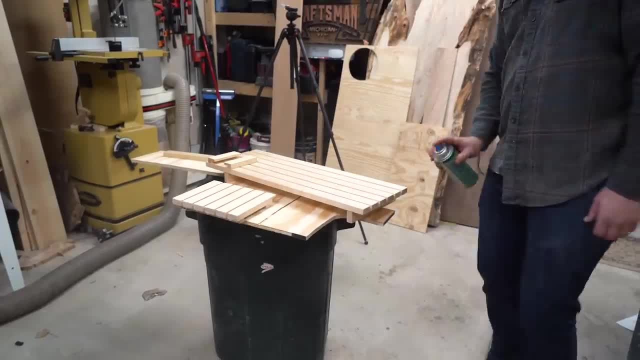 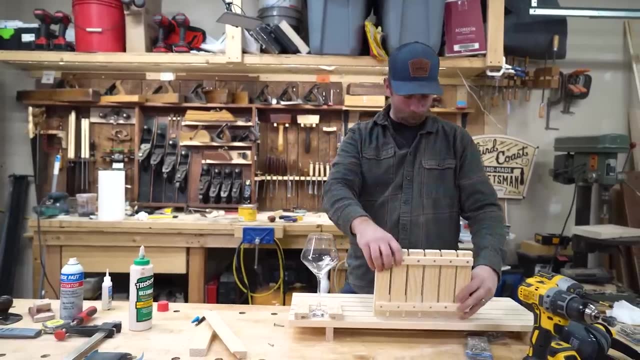 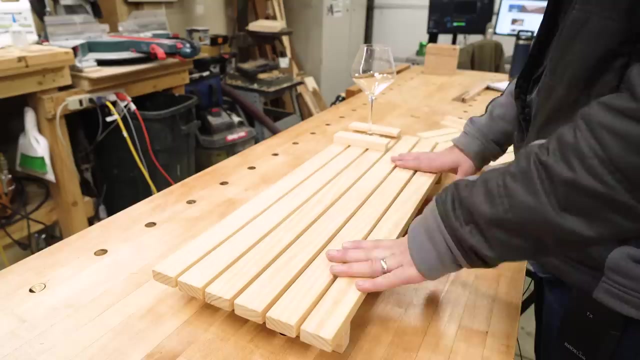 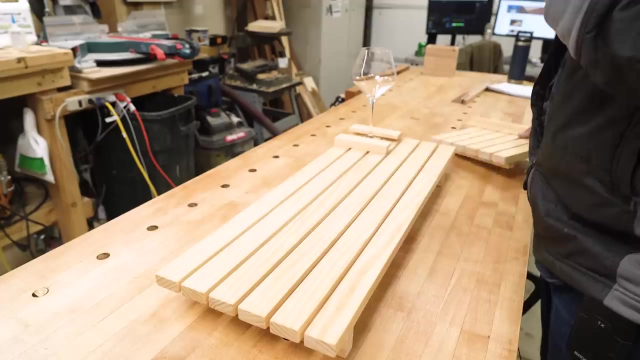 used to hold a wine glass. Then to finish the tray, I went with a Minwax spar urethane because of its great durability against moisture. So I wanted to make this little bathtub tray modular so you could remove parts of it. Can't remove this, this is glued and screwed down. but if you want to have 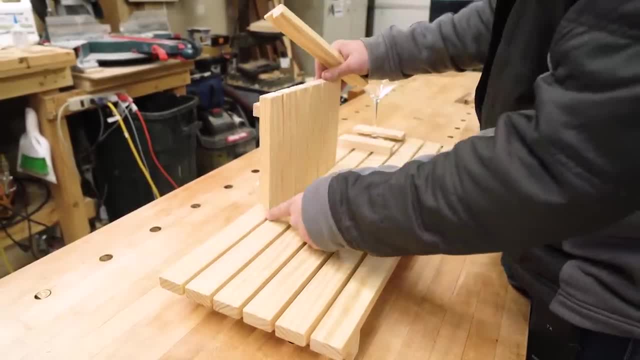 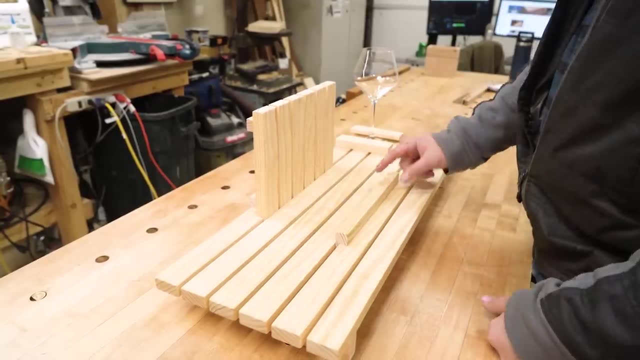 a book up there or your tablet. you can put this little piece in. It's a quarter inch to fit in the slot back there, and then also this little stopper piece that you can put in any one of these slots and then you could throw your book up. 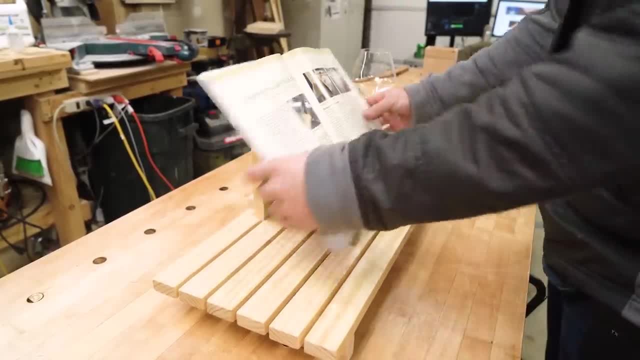 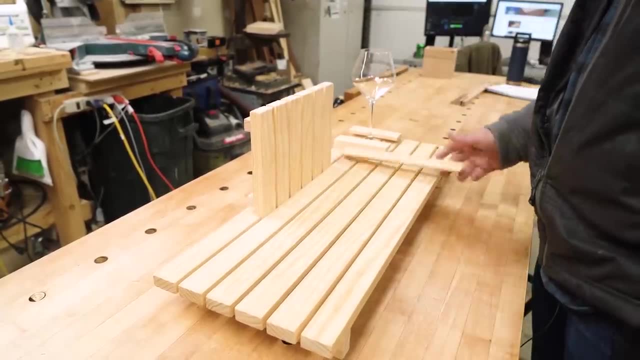 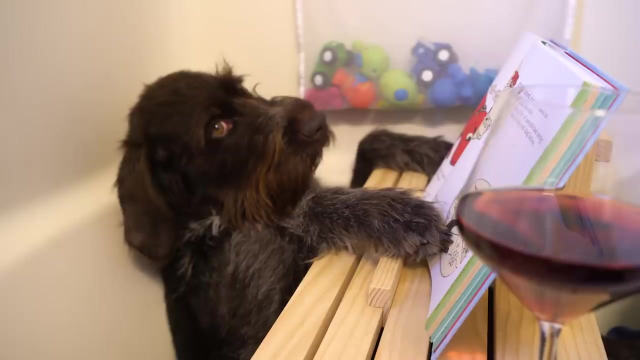 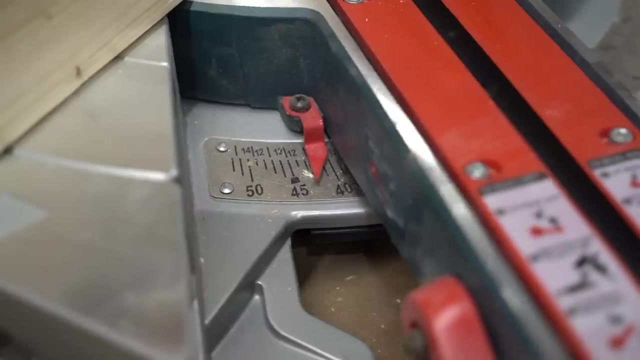 there and it'll hold it in place while you read. Or if you want to have a meal, if you like to eat in the tub, then you could take these off and put your plate on there. Okay, so this next project is super easy. It's literally just two 45 degree cuts. 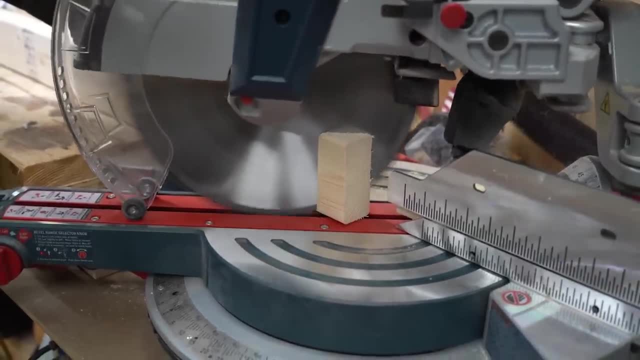 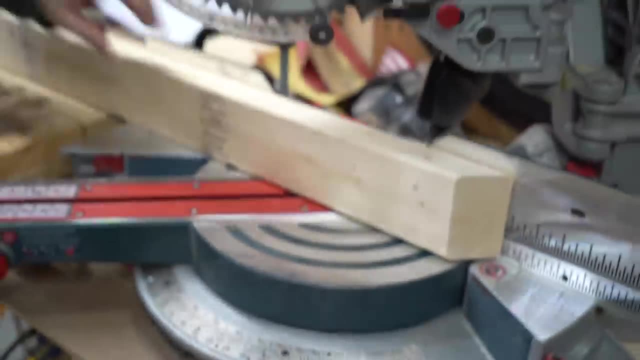 that are eight inches apart, and then a one and a quarter inch hole that's drilled five and seven eighths up from the bottom and just like that you have one of those really cool balanced wine bottle holders. I've seen some of these floating around the internet and I thought they were really neat. I've always wanted to. 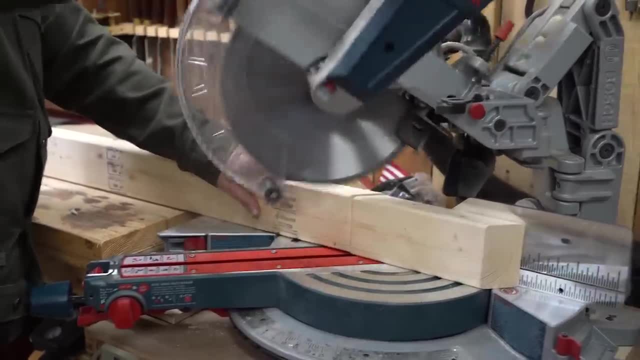 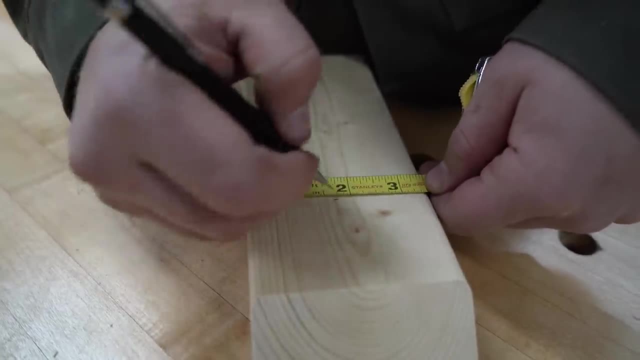 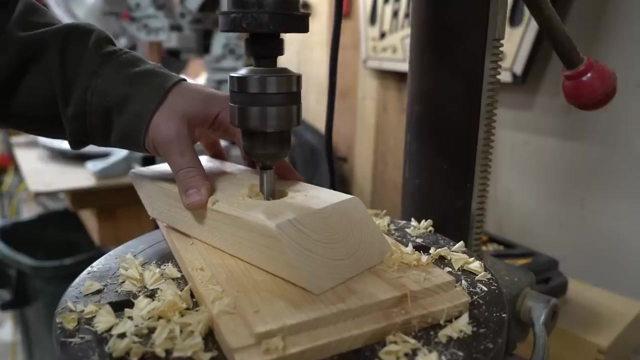 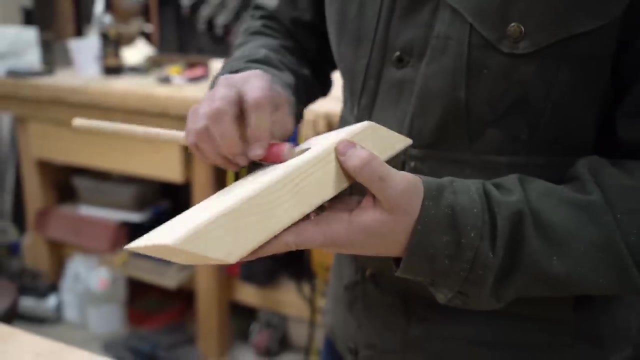 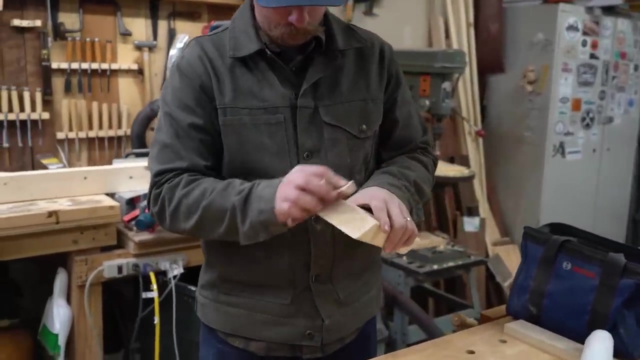 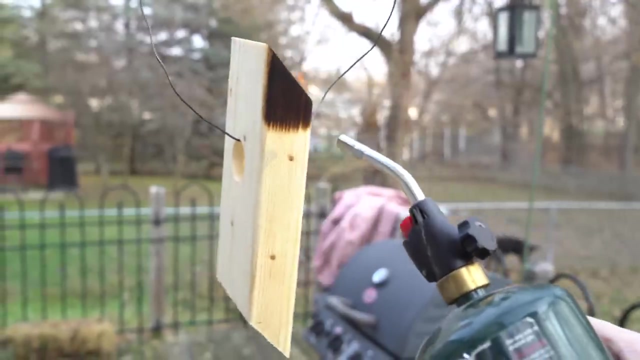 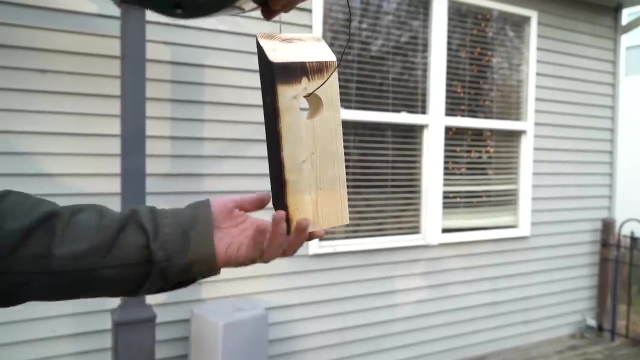 try making one, so looked up how to do it. It's super easy and will make a really good quick gift for somebody. Another technique I've always wanted to try is that shou sugi ban, where you basically burn the wood and scrape off the char and it leaves a really cool nice. 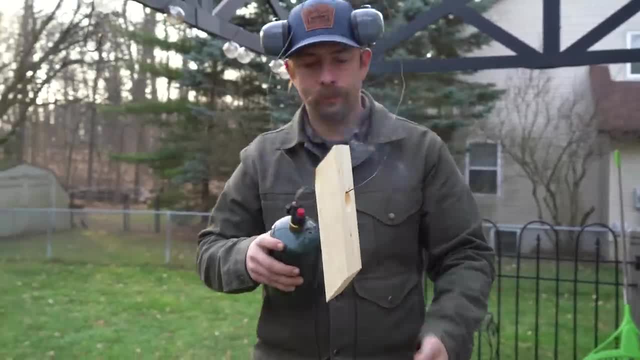 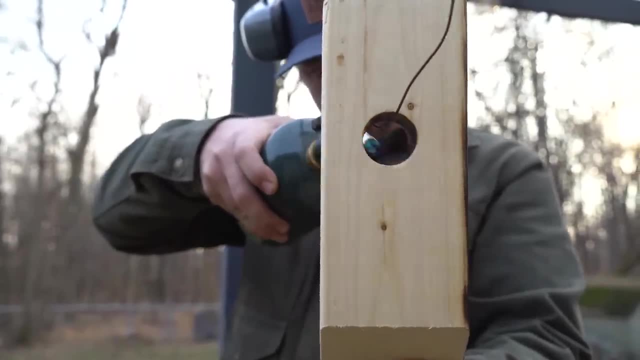 amber brown finish that's really durable. actually They use it in a lot of outdoor furniture and siding and it's an old, traditional Japanese method and then you add a little bit of Danish oil and it made a really nice finish. I thought it was a. 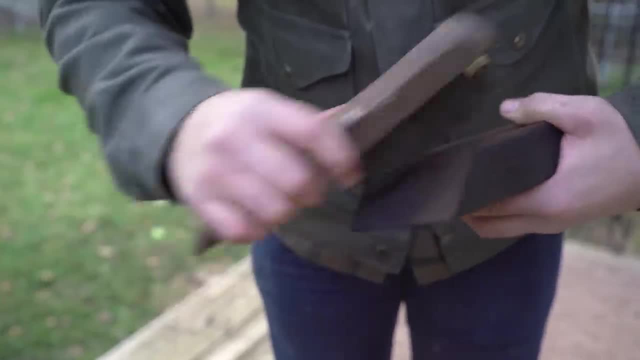 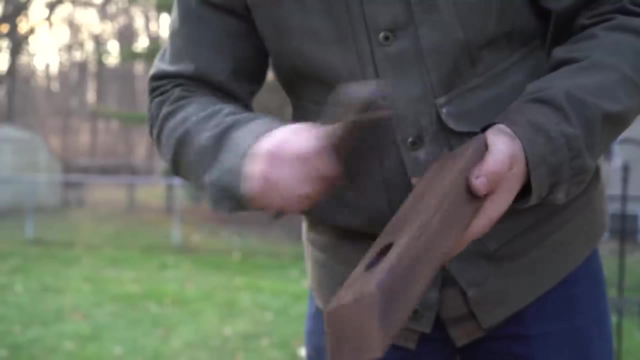 cool technique for sure. I used the three-point sandpaper and I'm just going to make tight people. I have a lot of dollars, but I'm trying to make something great with this piece. so what I'm going to do is I'm going to test this out, and I'm just going to try it out. 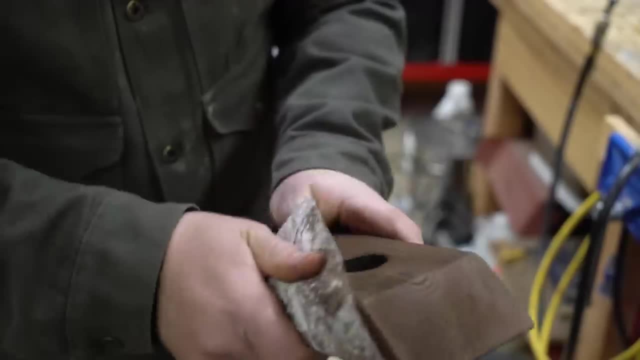 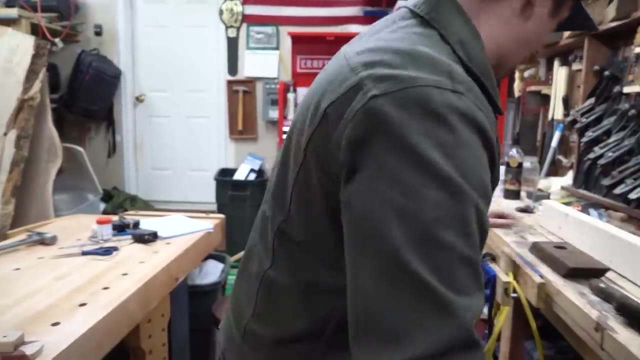 here and see how it goes with this water brush. so I'm just going to do that. Here we go. Here's what it looks like. You can see the little fingers and the little dots which are the letters for the pen. You can see that I'm using a wooden brush here. 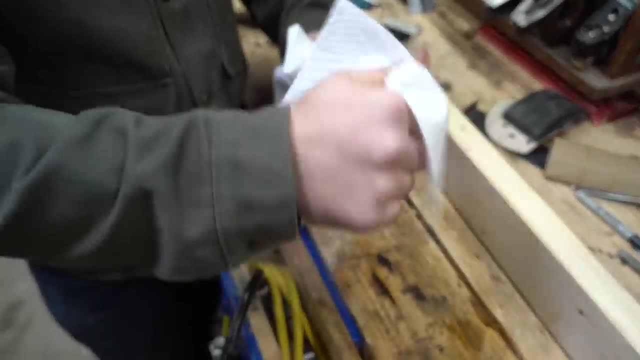 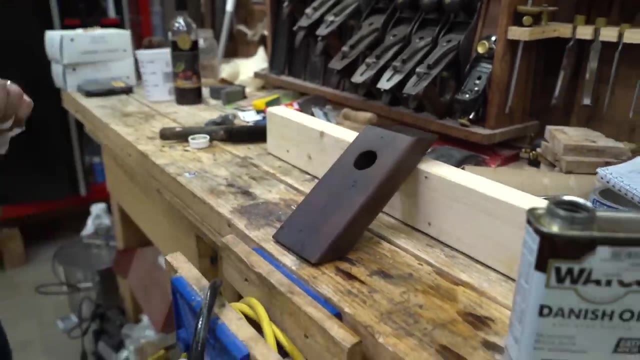 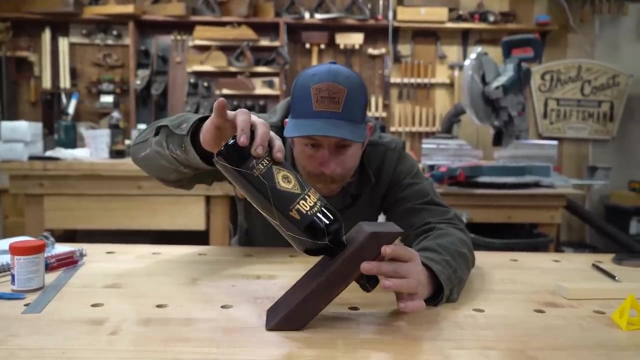 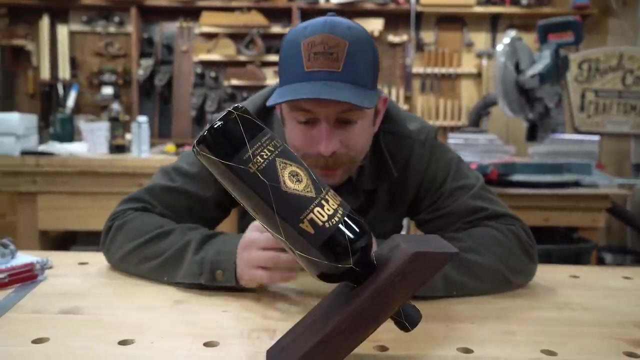 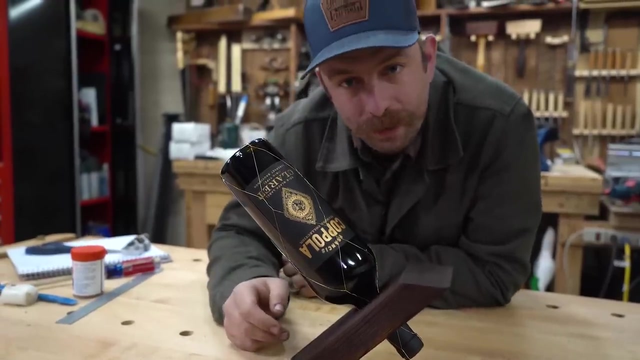 And then I'm going to mask that in on the wood here so you can see the difference. Voila. there's no better way to display your beautiful bottle of wine than through a 2x4.. But actually you can make these out of all sorts of cool things, like exotic woods maybe. 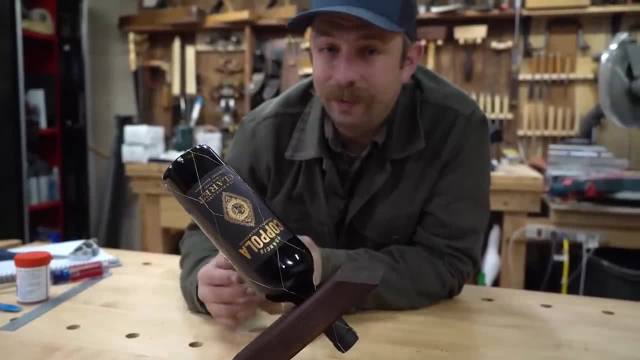 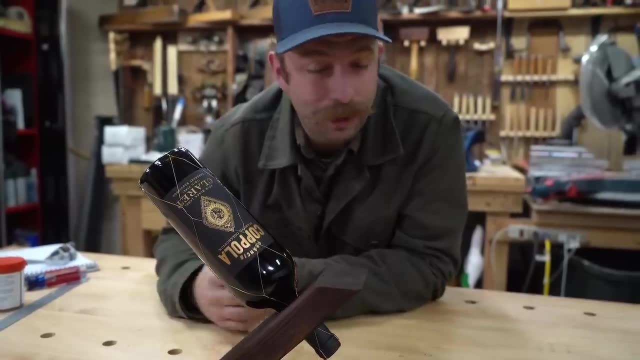 a live edge piece. it doesn't have to be a 2x4,. the wider the base is, the more stable it's going to be. But you can do it out of narrower pieces of wood. The possibilities are endless, so have fun with that. just follow those dimensions and 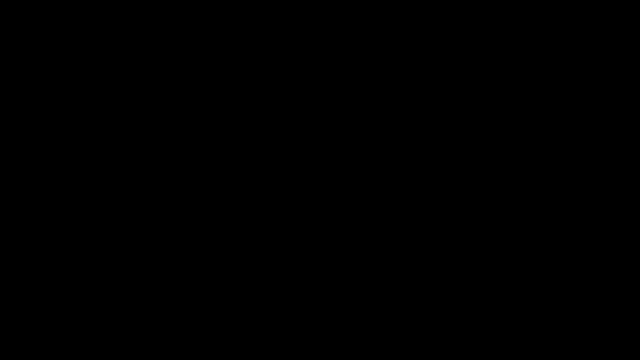 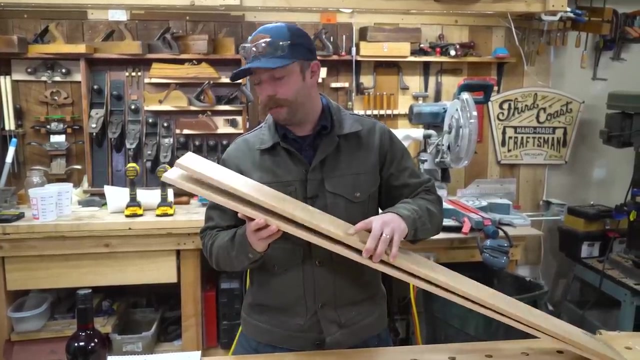 you'll be able to make all sorts of cool little, super easy gifts. Alright, now we're going to make a nice little wine gift box. Now, Lowe's had a couple of oak boards that were already dimensioned, so these are half inch. These are quarter inch boards for the lid. 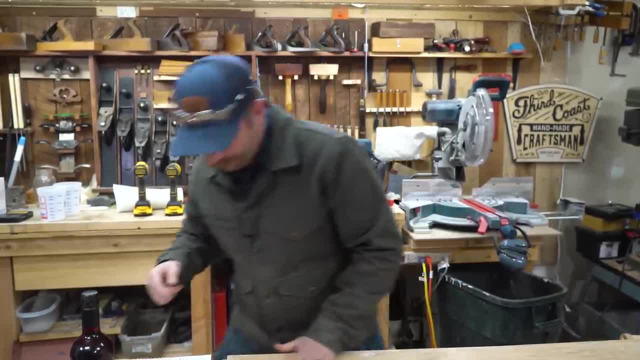 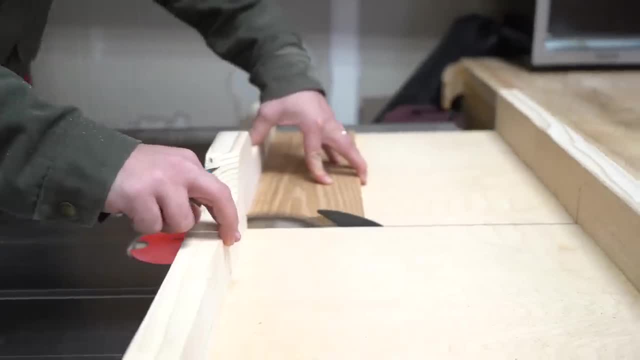 We're going to do a little bit of a ducktail joinery on it, So let's get started. The first thing I'm going to do is cut all my boards to their final length and width, and instead of trying to explain it all here, I'll just put those measurements down in the 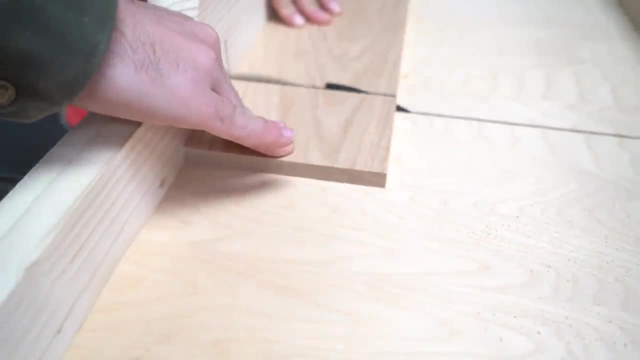 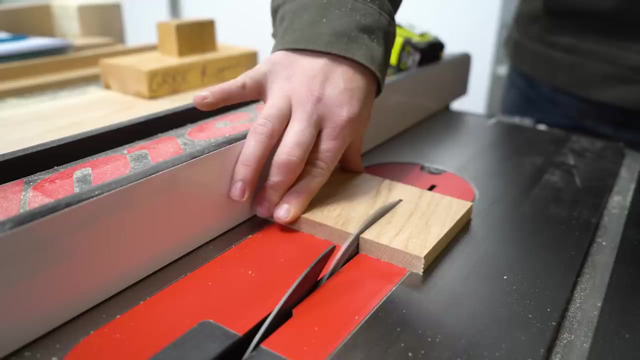 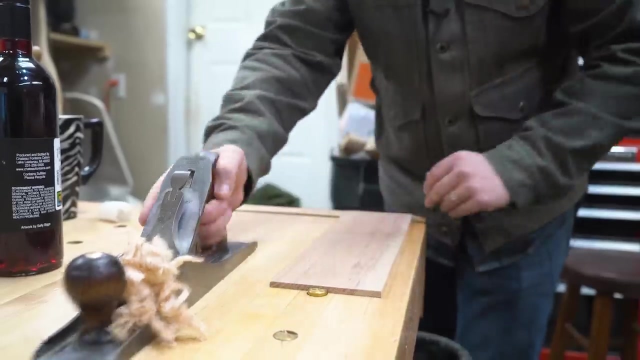 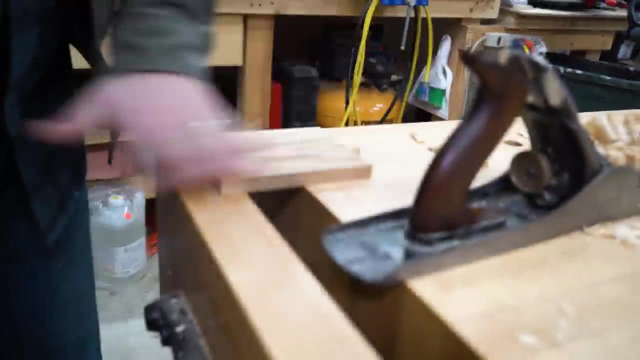 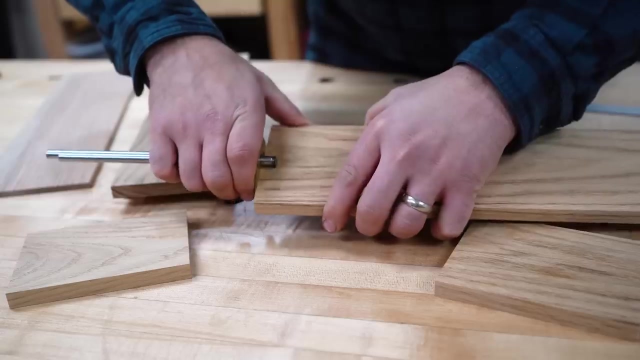 description: These boards are milled up really nice already, but I still wanted to take a couple passes with the hand plane to give them that ultra smooth finish. You could also touch them up with some sandpaper too, if you wanted. I haven't cut any dovetails in a while, so I decided to challenge. 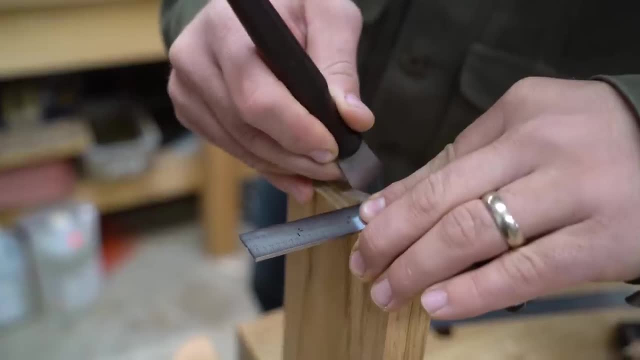 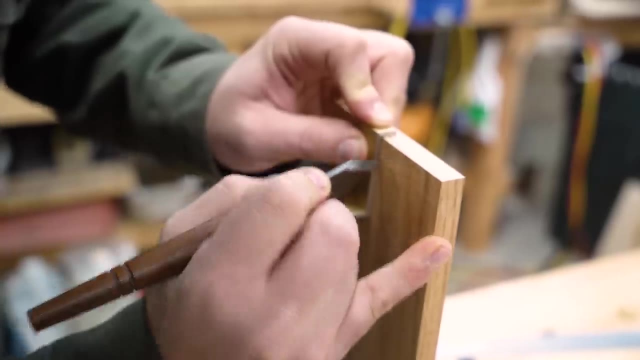 myself with those for this project. but this box could be joined together using box joints, miter joints or even just butt joints. with some glue and brads, The box will still look good and be plenty strong for what its purpose is, which is just holding a bottle of wine. 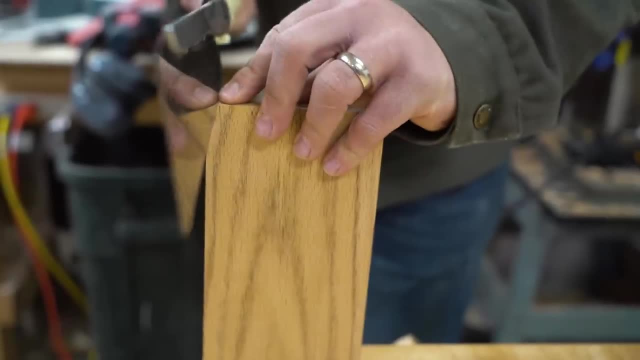 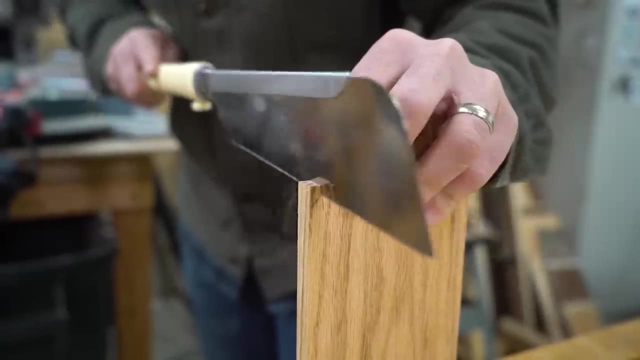 So I lay out my dovetails on what are called the tailboards. first, I like narrow, delicate looking dovetails, so I lay mine out to look like that and using a Japanese pull saw, I'll do my best to cut right on the waist side of the line. Then I'll use my fret saw and chisels to get rid. 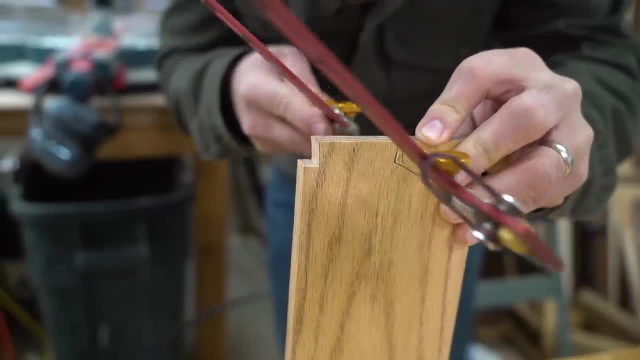 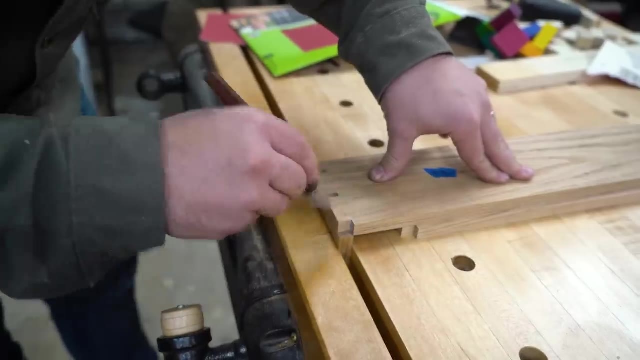 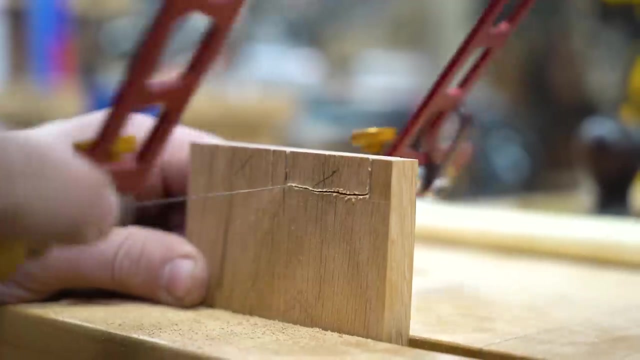 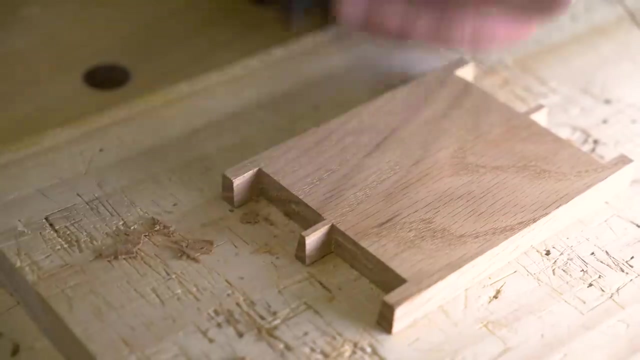 of the waste. Then, using the tailboards and a marking knife, I can mark the ends of the dovetails and mark out my pins board. And again, I do my absolute best to cut just to the waist side of the line, leaving barely the line visible. And if I'm accurate here, I won't have to do any tuning. 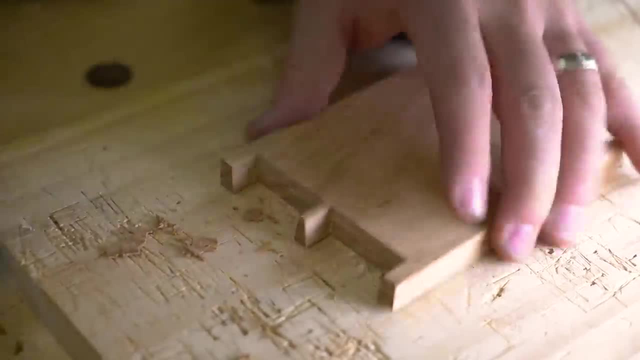 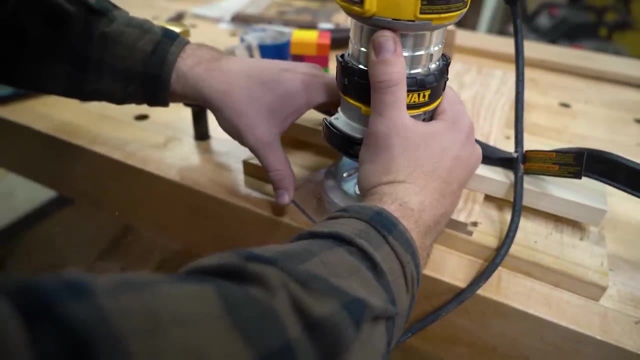 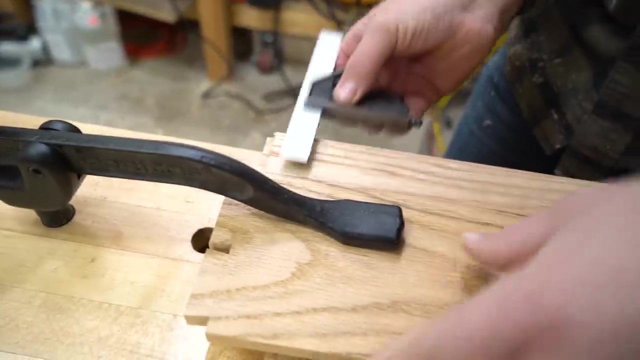 with a chisel and I can get a nice tight joint just from the saw. Then, using a router and clamping a fence on my bottom board, I'm going to cut a rabbit that will then later on sit in a dado that I'll cut on the side and front and back pieces later on. But to save yourself this, 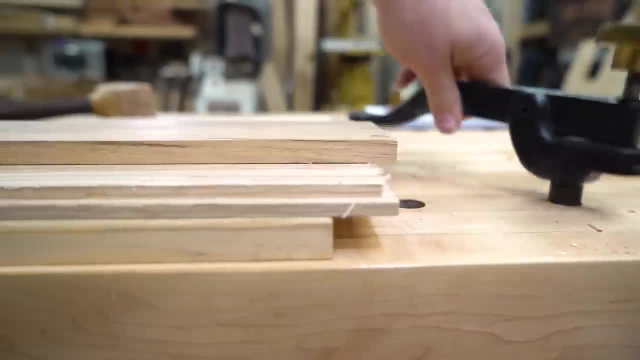 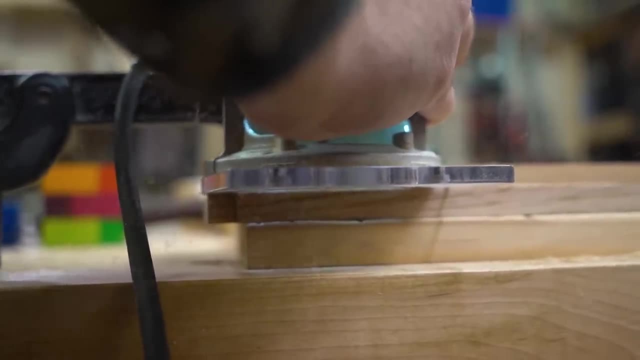 step. you could just use a quarter inch piece, like I used on the top. I would probably do it that way next time. Now, using a quarter inch spiral up cut bit, I'm going to cut dados in the tops and bottoms of the box frame pieces so that the bottom can sit in and the top can slide. 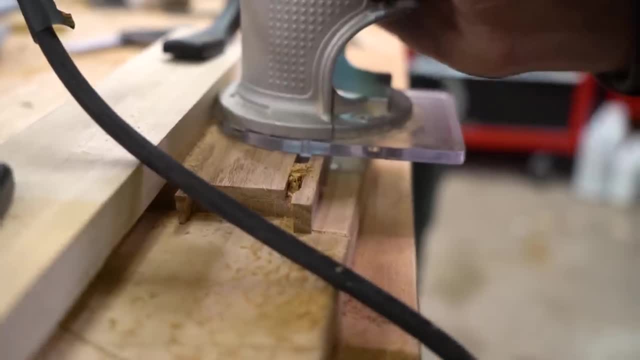 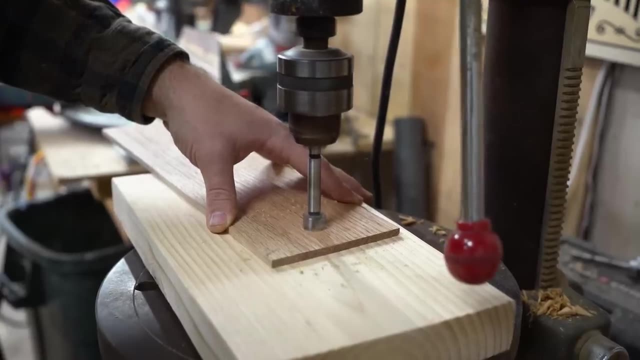 into. I make sure that I don't go all the way through the cut and stay about a quarter inch away from each end, so it's not visible through the dovetails. Next I'll make the lid using a quarter inch thick piece. I'm first going to drill a three quarter inch finger hole that I can use. 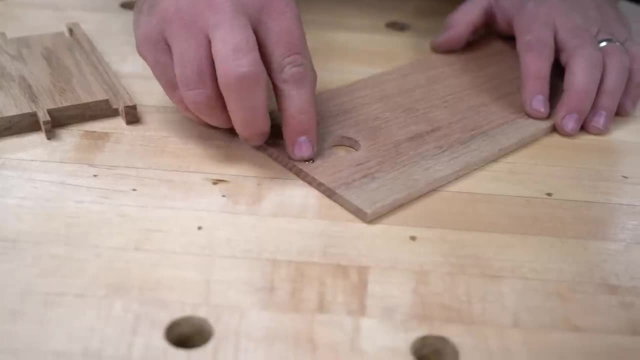 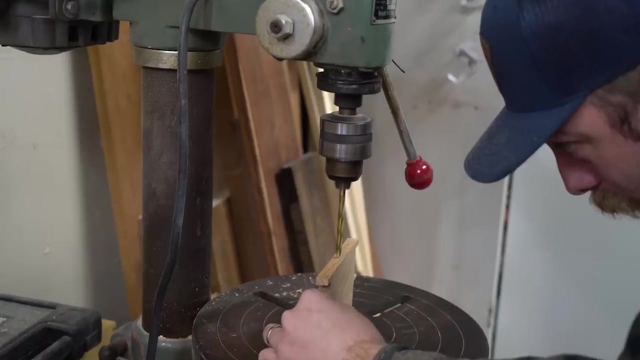 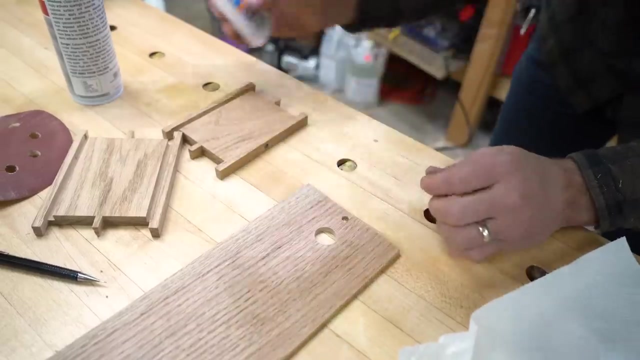 to open and close the lid, then a small quarter inch hole that I'll use to embed a magnet in to help keep the lid closed. Then I'll drill a hole and add a magnet to the front piece before I assemble. Then I'll scratch the surfaces of the magnets with some sandpaper to help the glue grab. 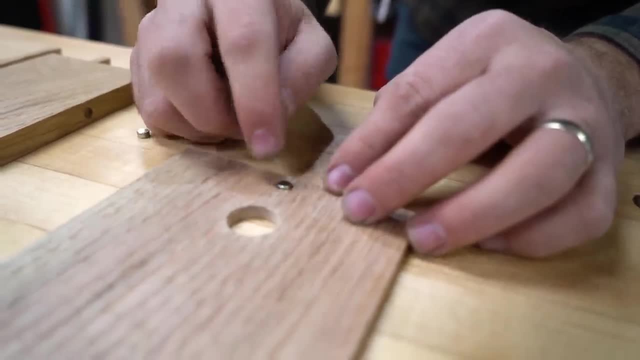 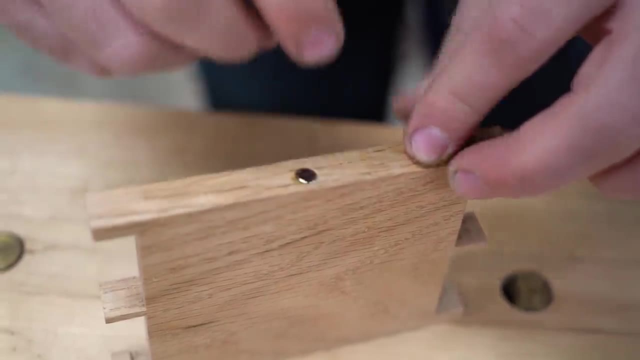 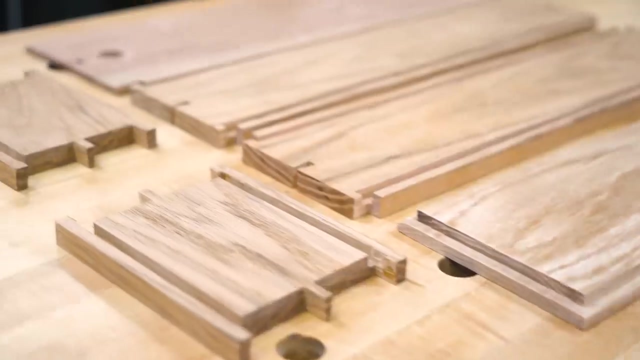 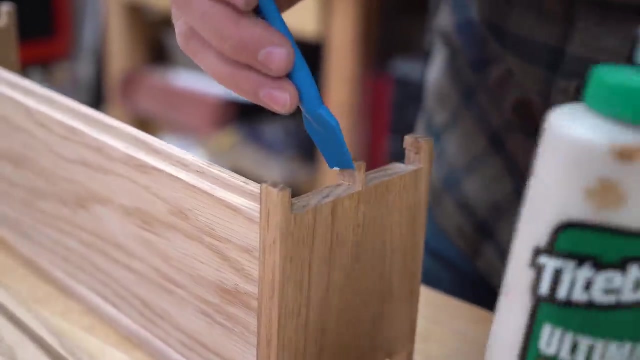 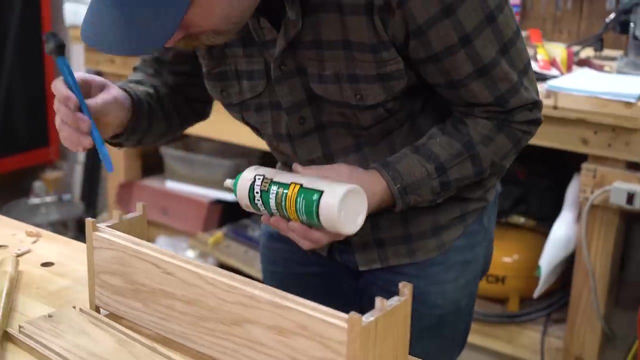 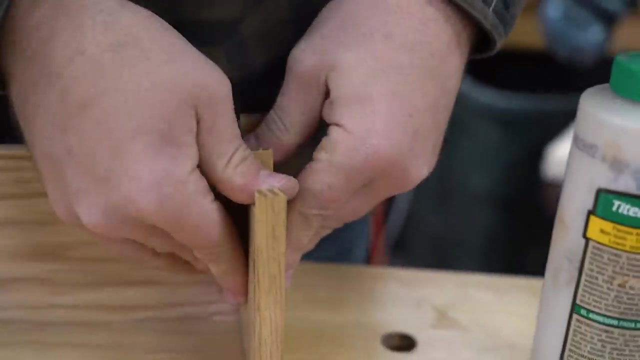 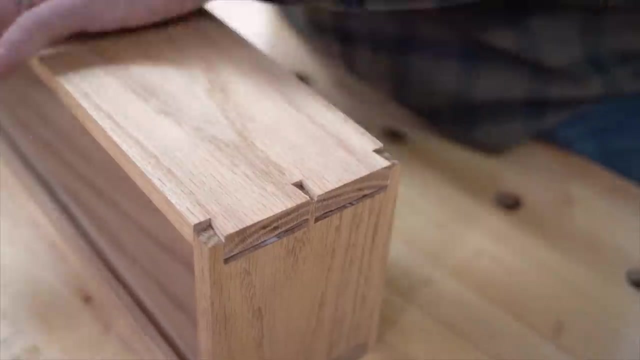 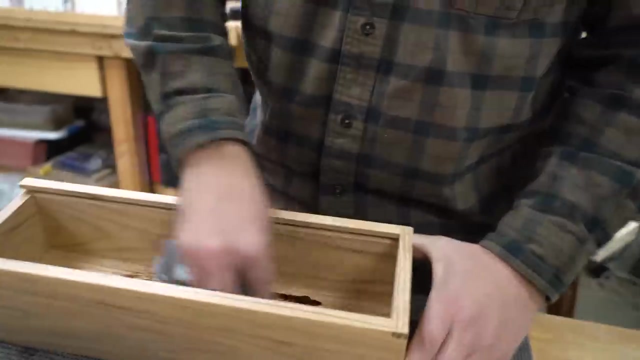 and I'll use some CA glue and instantly bond it using a shot of activator. Then I add some glue to the pins and assemble the box. I decided to add some finish to this box and I went with some Minwax Red Mahogany to try to give it a more aged, rich look. 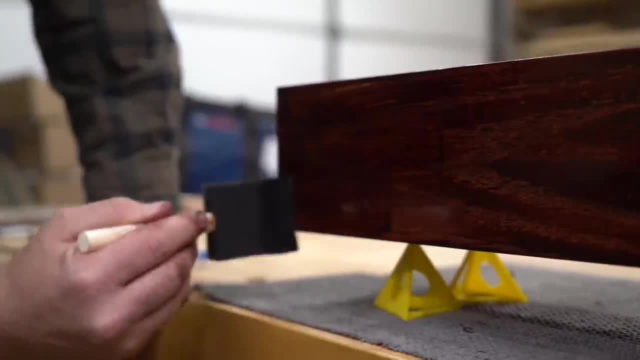 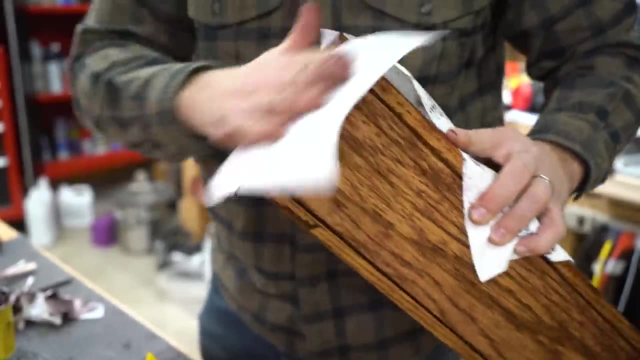 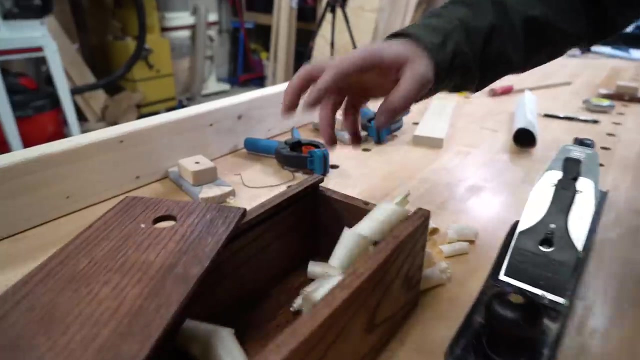 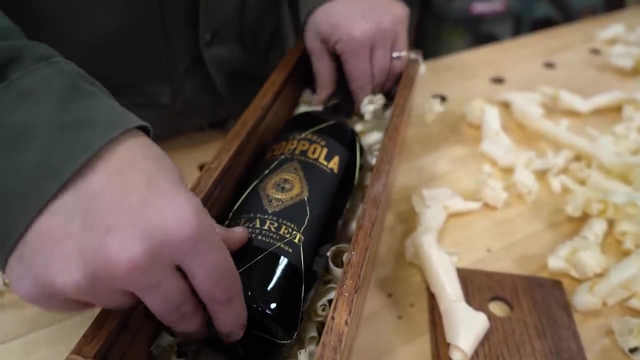 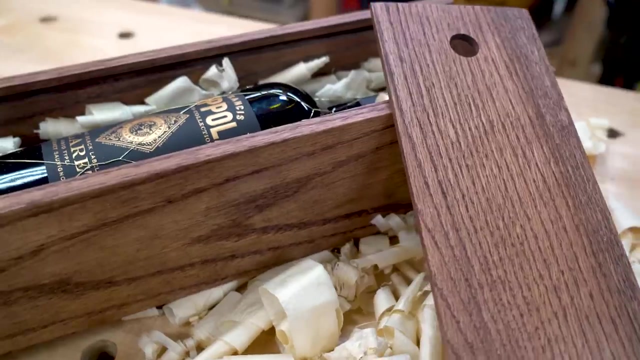 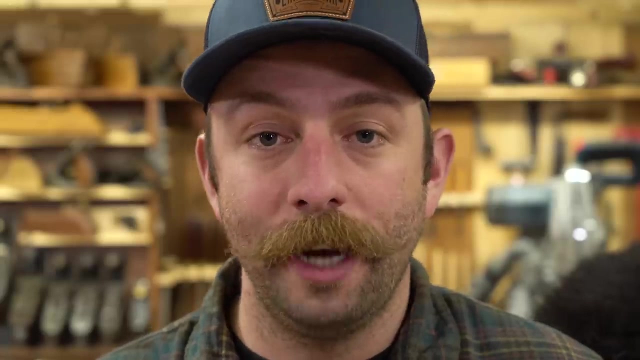 and I'm definitely happy with the result. Well, I'm super happy with how this little wine box came out, and I think it's a great way to spruce up a somewhat ordinary gift. Alright, so now for the final bonus gift. This is actually a gift to all of you and my wife.